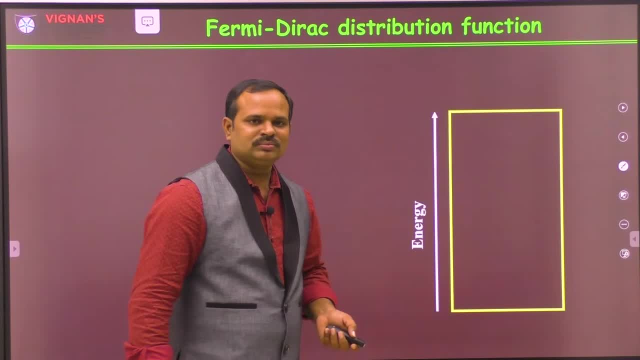 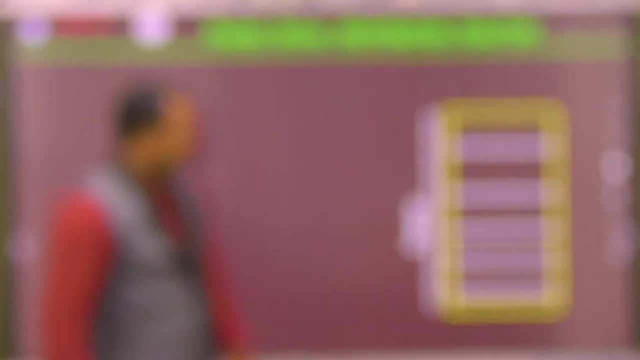 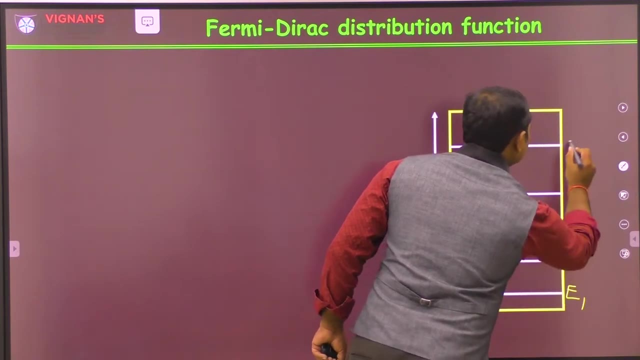 For example, this is a quantum mechanical system. So quantum mechanical system means the energy levels are discrete, like this way. These are all discrete energy levels. with energy, This is it: E1,, 2,, 3,, 4, 5 and so on. 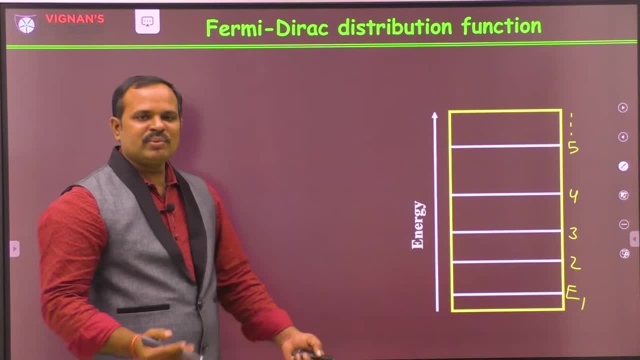 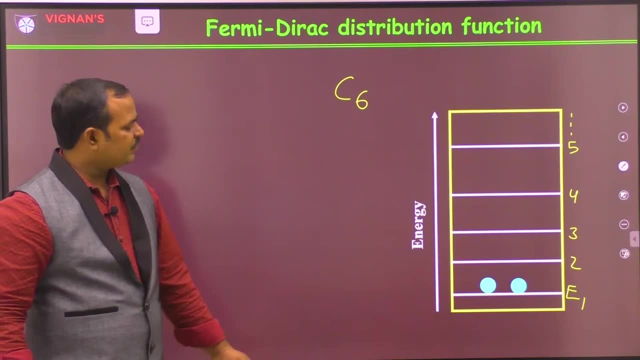 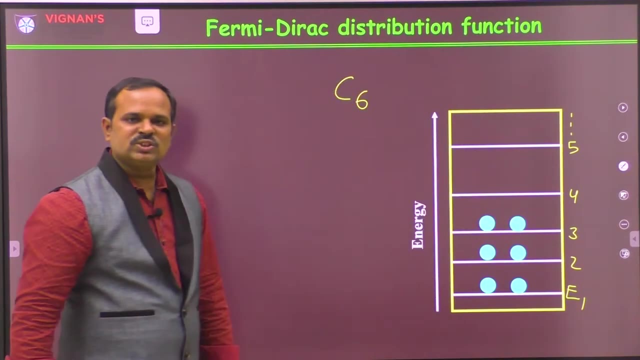 Now, if I have a 6 number of electrons, like for example, a carbon atom, Now these electrons are distributed like this way, and so on. So this follows a Pauli's exclusion principle and Hounsoul. This we have seen in the last class. 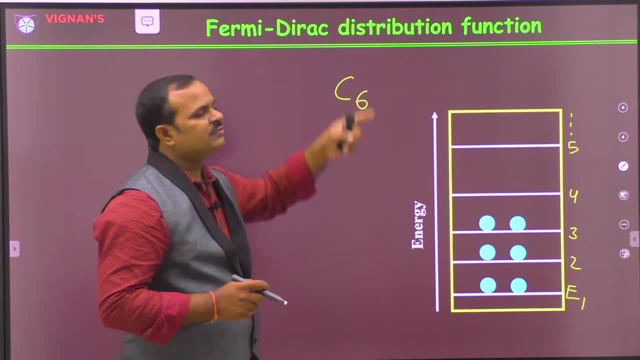 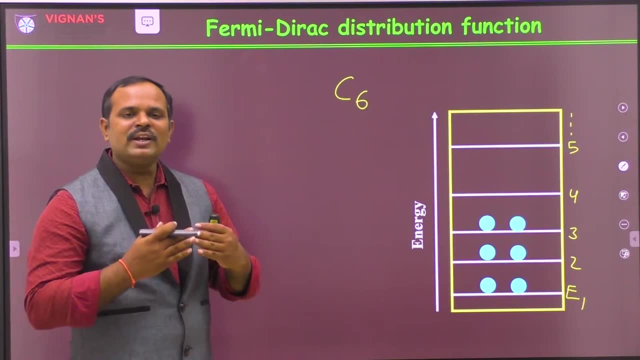 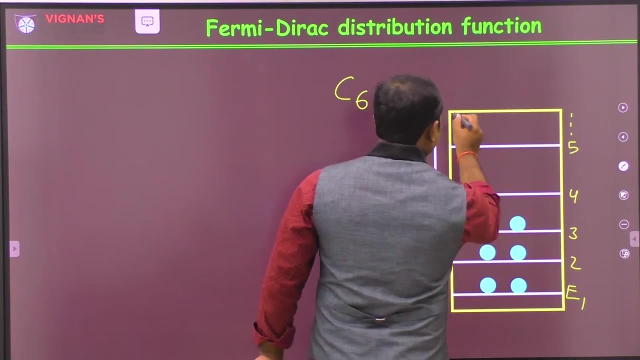 Now, what is the distribution? Fermi Dirac distribution function tells us the probabilities of finding the particle in any energy level. I have so many energy levels. I have shown only 5 energy levels here, but I can have n number of energy levels continuously like this way. 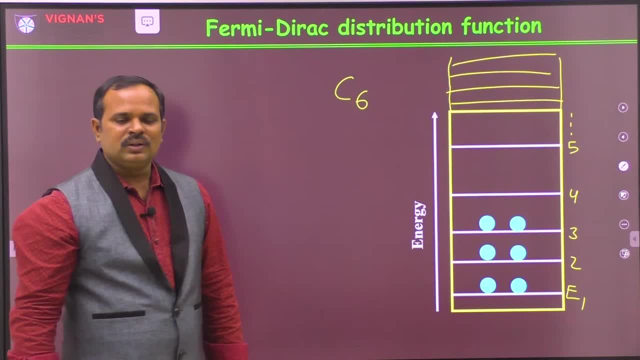 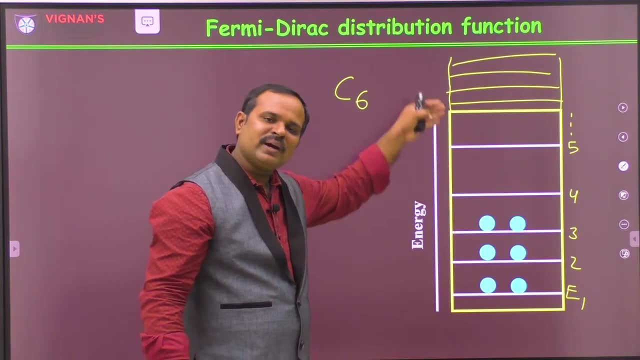 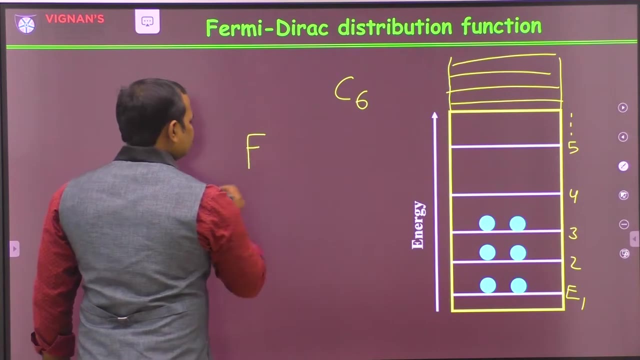 There will be so many energy levels in any system, How to find out the presence of one particle or an electron In any particular energy level That one is given by is going to be given by Fermi Dirac distribution function f of E. 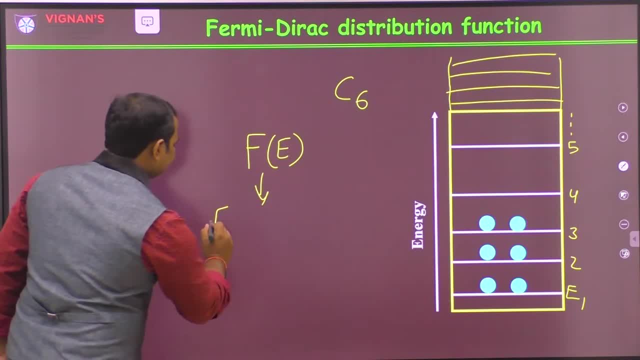 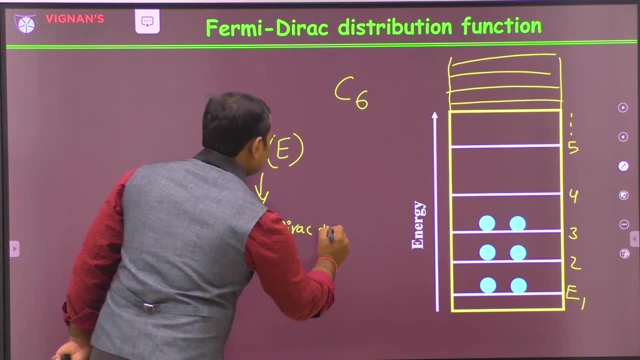 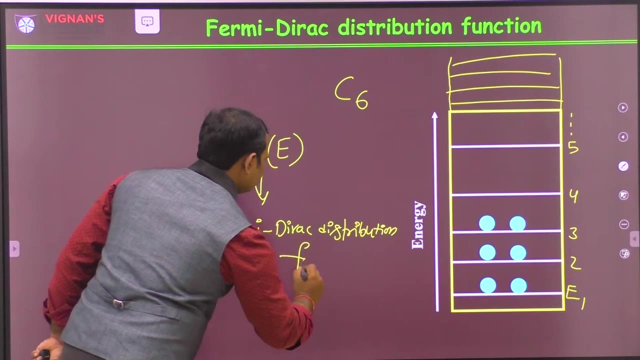 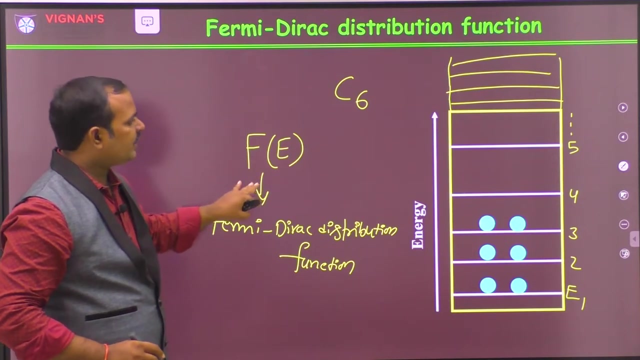 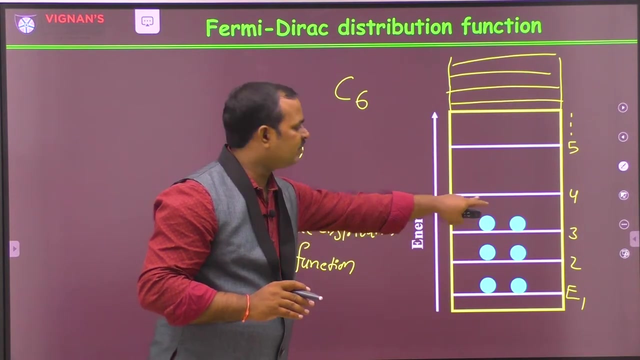 This is the Fermi Dirac distribution function. This is the F of E is a Fermi Dirac distribution function. It can give you an information about how, where the electron is present and, for example, if you take a particular energy level, fourth energy level- if there is any particle or electron is present in this particular. 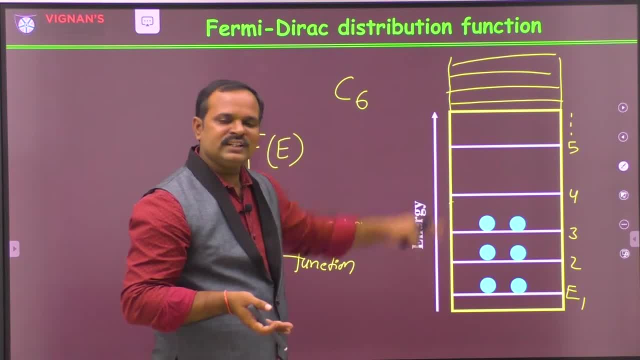 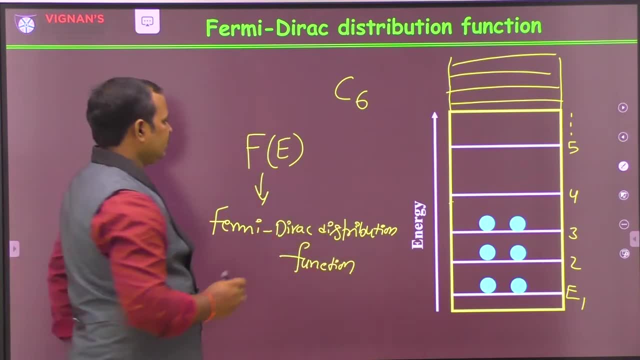 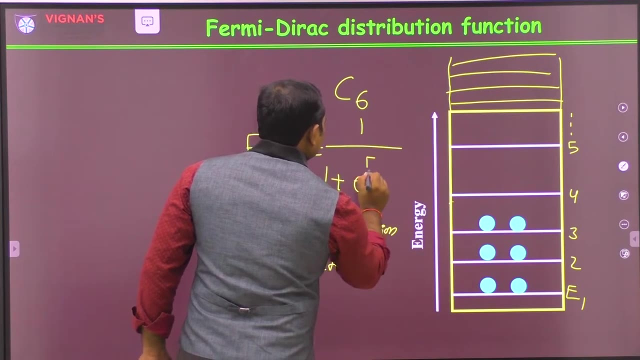 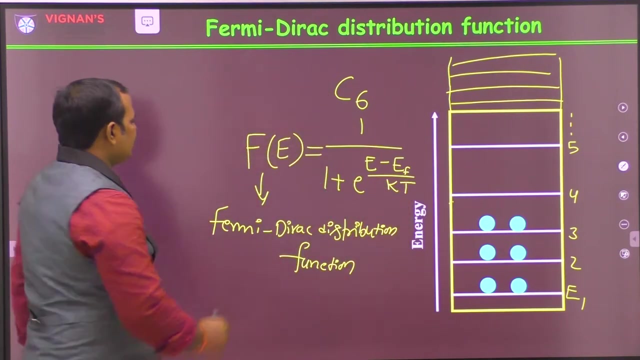 energy level or if you take any other level out of all these things. if the particle is present in a particular energy level, then this function can give you an information. in this way: F of E is equal to 1 by 1 plus E power, E minus EF by kT. This is the Fermi. 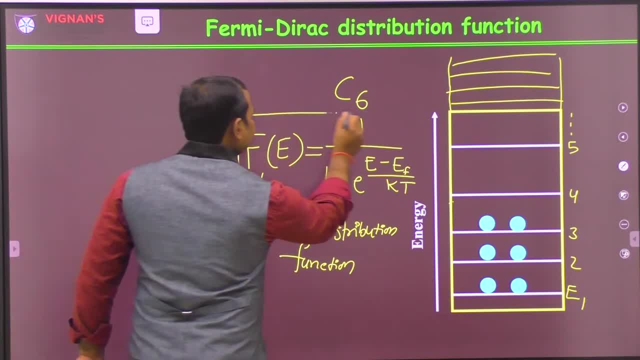 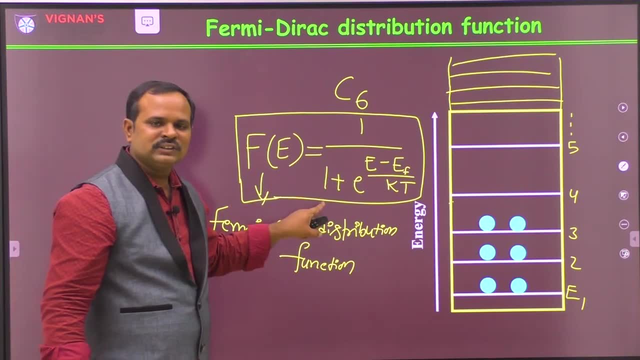 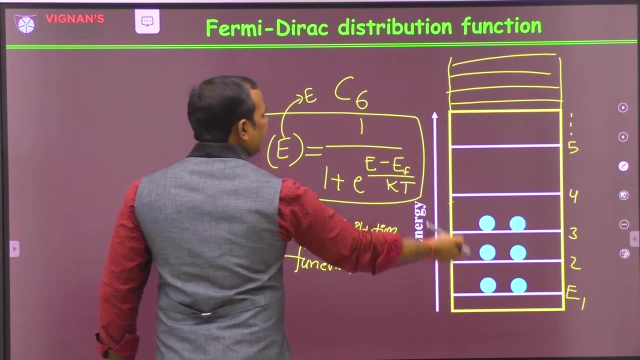 Dirac distribution function. This is the Fermi Dirac distribution function. This function can tell us if the particle is present in a particular energy level of energy E. This E could be anything E1,, E2, E3 and so on- anything Here EF is called Fermi energy. 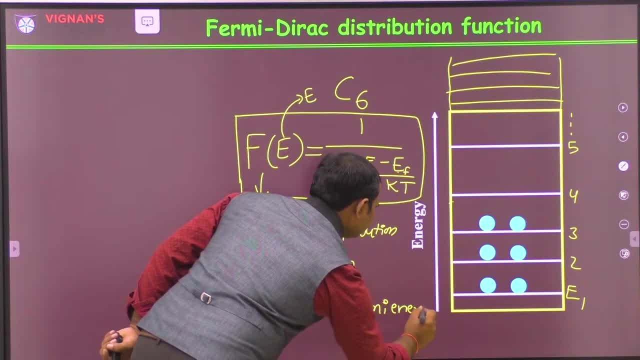 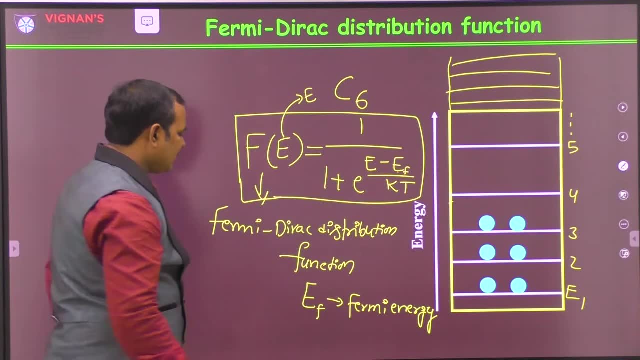 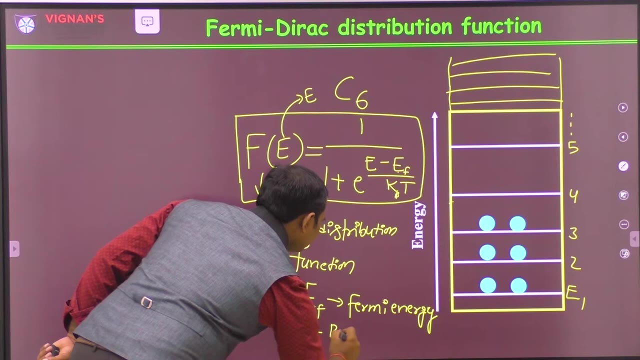 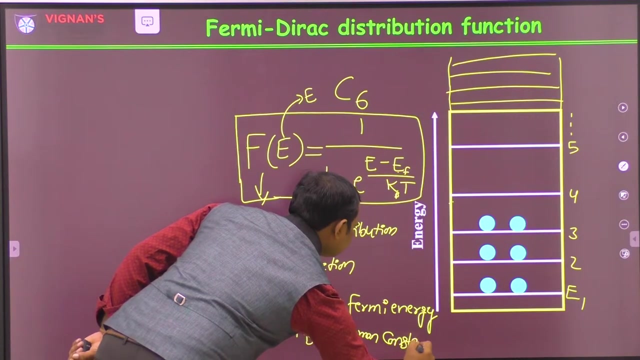 EF is called Fermi energy level. We will see that. what is the Fermi energy level? ke is the Boltzmann constant, kb. Actually this is a, b should be there, kb is the Boltzmann constant and T is the temperature. 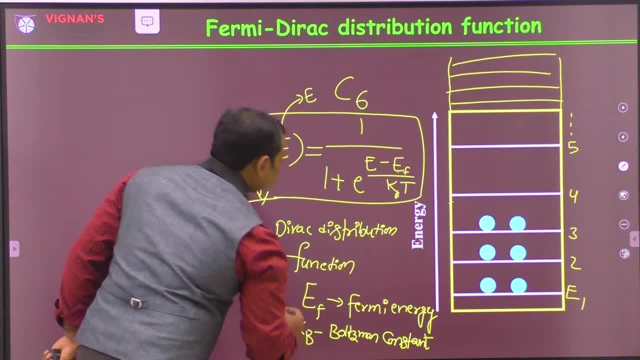 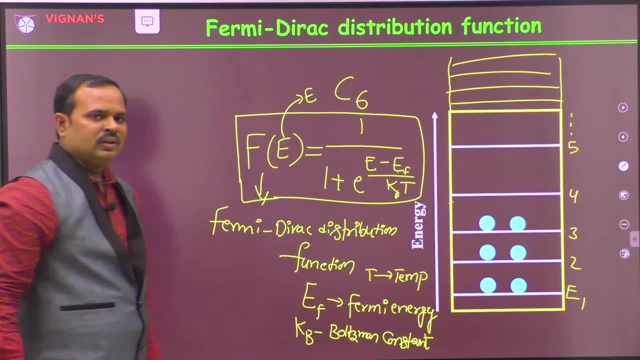 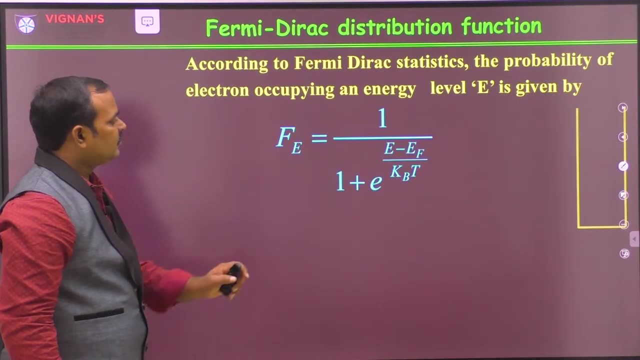 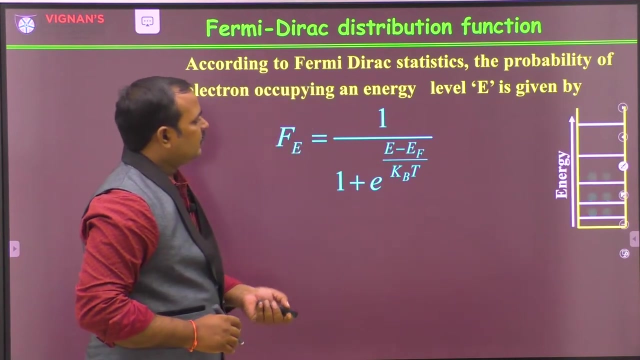 Thank you for watching. Now, how does? this gives information. Let us see. This is the Fermi Dirac distribution function. those are the energy levels we have already taken. Now, this is the energy levels let us consider. this is the first energy level. this is second. 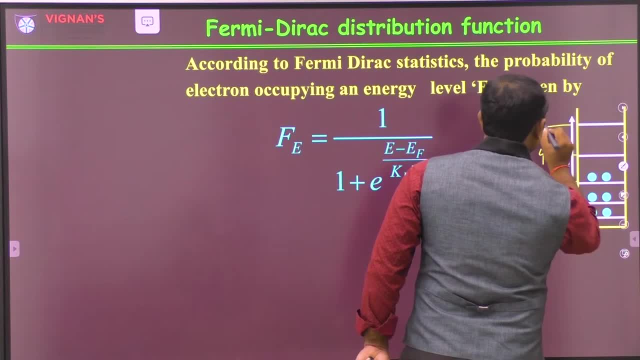 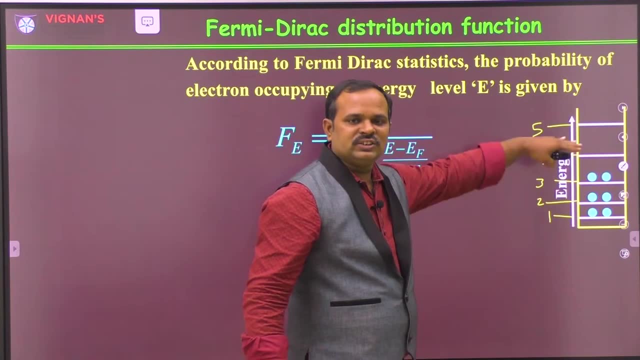 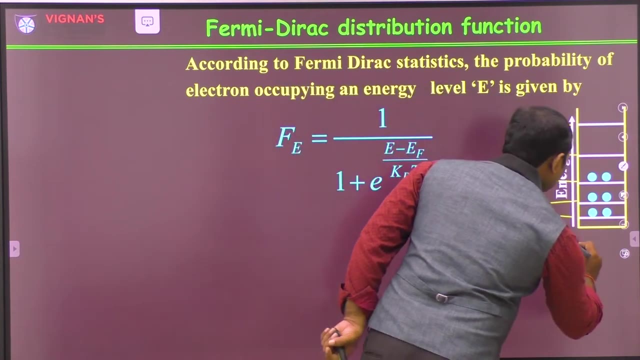 energy level. this is third. fourth, this is the fifth, as per the increasing energy order. Now this is how the six electrons are distributed according to Hounsroll and Pauli's exclusion principle. Now, if you consider at, T is equal to T, zero kelvin. we are taking an example at absolute. 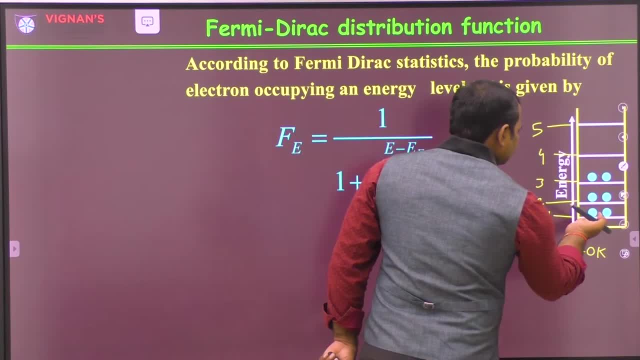 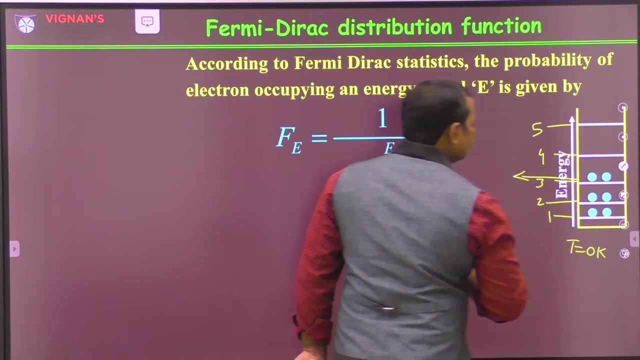 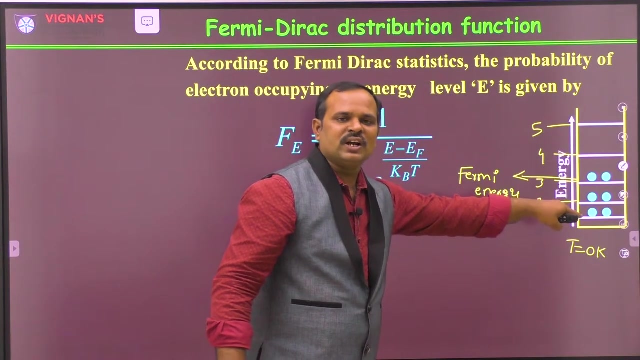 zero kelvin. Now the electrons are distributed in this energy level, The topmost energy level, The topmost energy level, which is a field energy level, is called the topmost field energy level, is called Fermi energy level. At zero kelvin, the topmost field energy level is called fermi energy level. 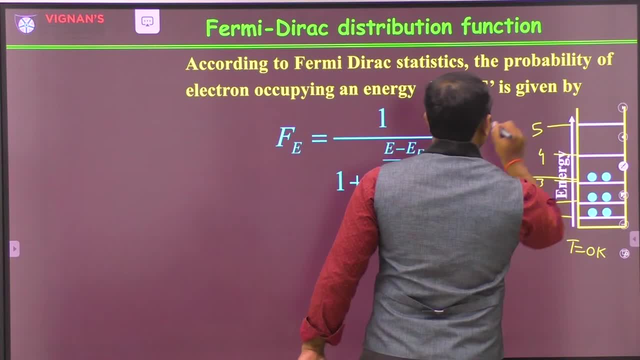 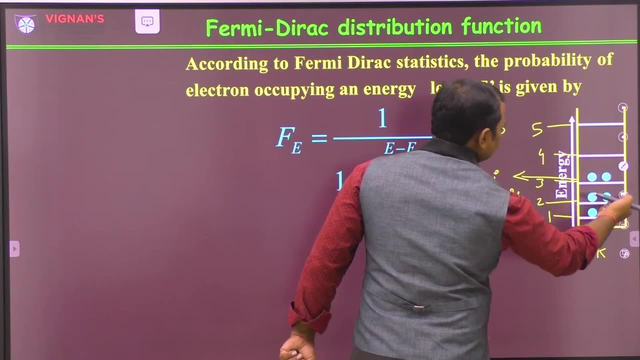 And you can see, at zero kelvin you have taken six electrons, that is a carbon. All these exact electrons are distributed in each energy levels: ms2, this is 1s2, 2s2, 2p2.. And this is the highest energy level which is filled at t. 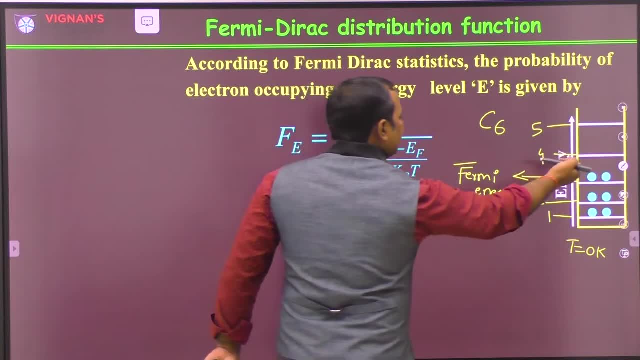 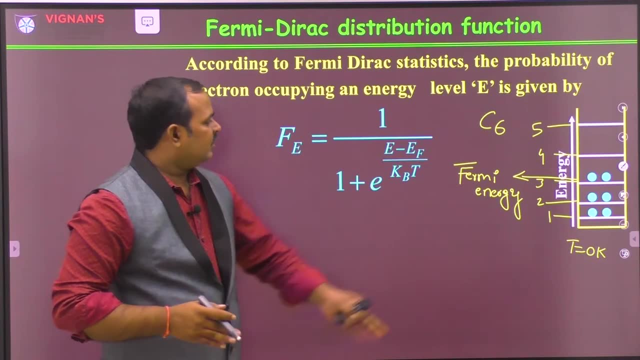 is equal to 0 Kelvin. This is called Fermi energy level And above which all these energy levels there may be, so many energy levels are there. All of them are empty and they are not filled by any electrons, because the electrons are completed by here itself. 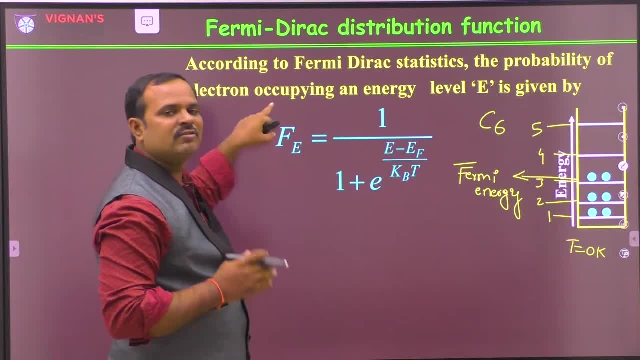 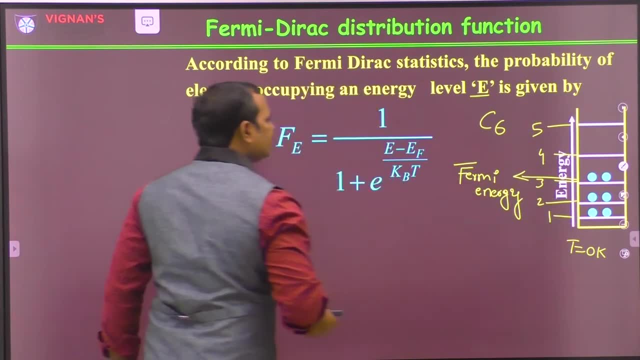 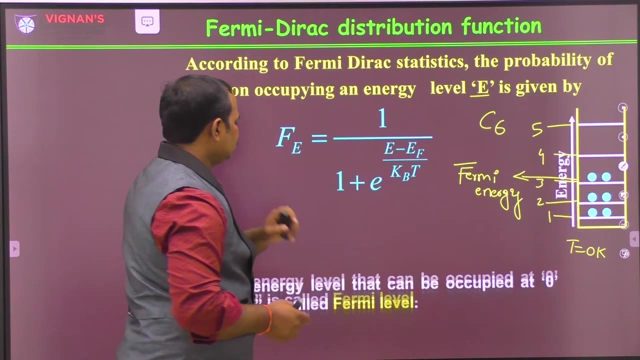 Now, if you see here the Fermi Dirac statistics, probability of finding an electron in a particular energy level, that energy level- E- it could be anything among these- is given by this. We have already seen what is E, what is EF, Kb and T, So the highest energy level, that 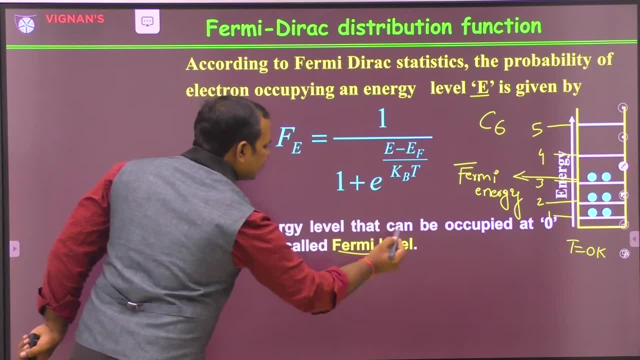 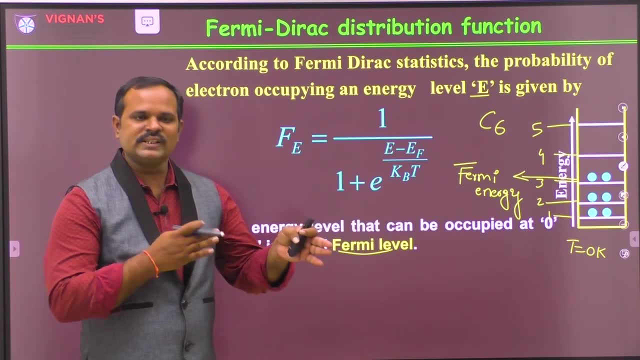 can be occupied at 0 Kelvin. 0 degree Kelvin is called Fermi energy level. This is the definition of the Fermi energy level. Fermi energy level has a lot of different definitions. You will see them as you go on. This is one definition. 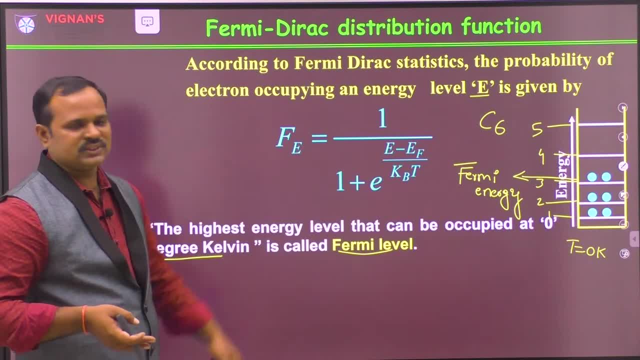 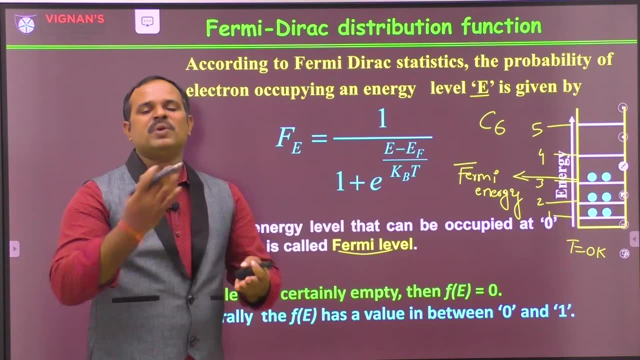 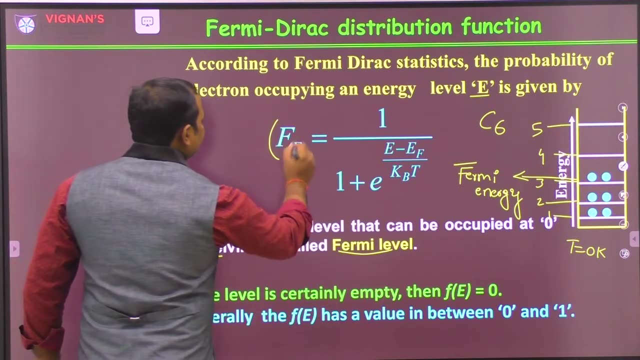 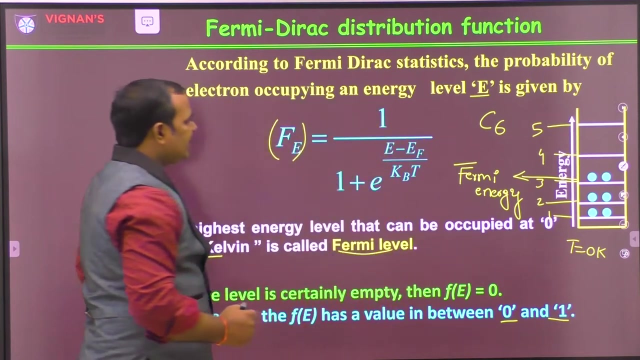 You will also see many other definitions. as per the situation- And this is a probability- in the quantum mechanics We always tell the probabilities. in terms of probabilities, The probability is always lying between 0 and 1.. So similarly, here also the Fermi Dirac distribution function also lies between 0 and 1.. And if there is 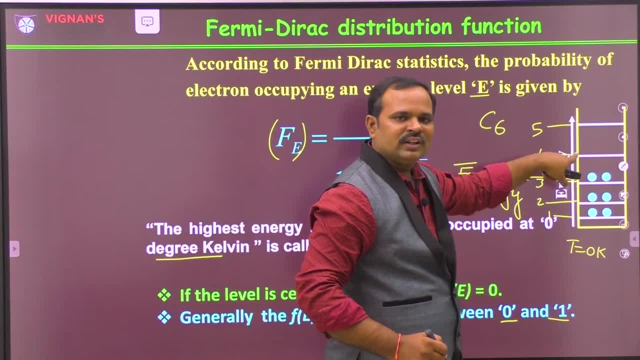 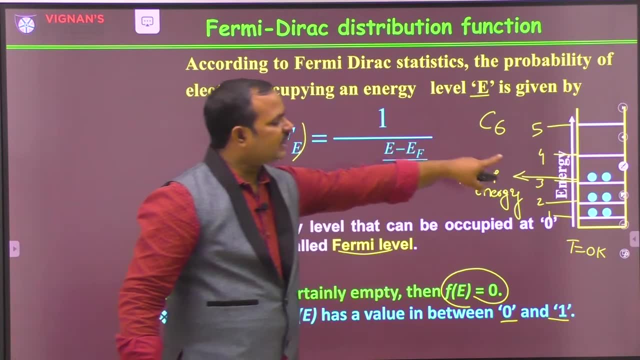 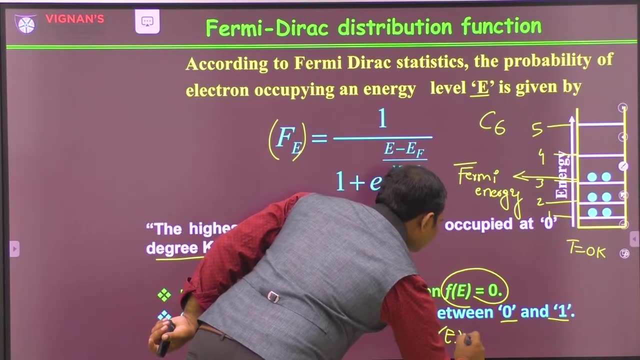 no particle. for example, if there is no particle in this particular energy level, then the Fermi Dirac distribution function gives a value of 0.. If there is any particular energy level, that particle is present or electron is present, then the Fermi Dirac distribution function gives you a value of one. 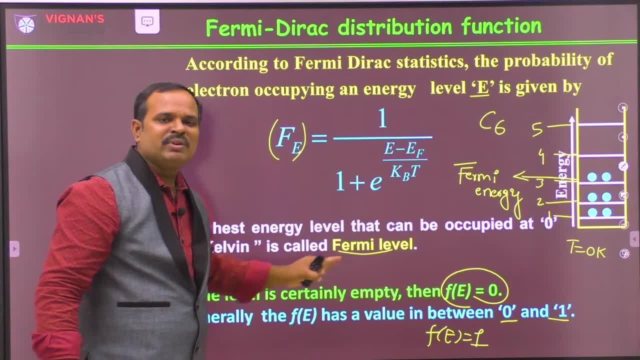 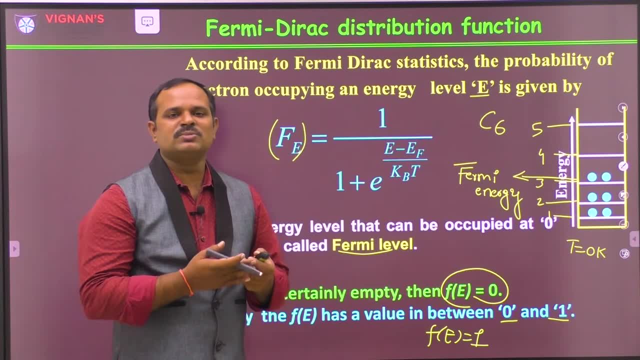 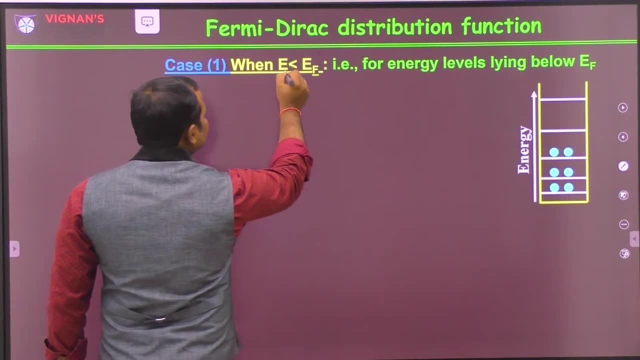 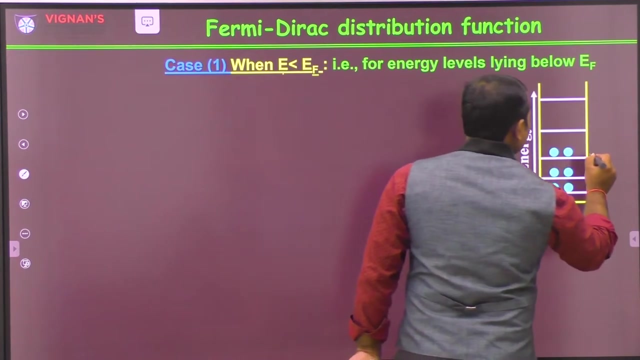 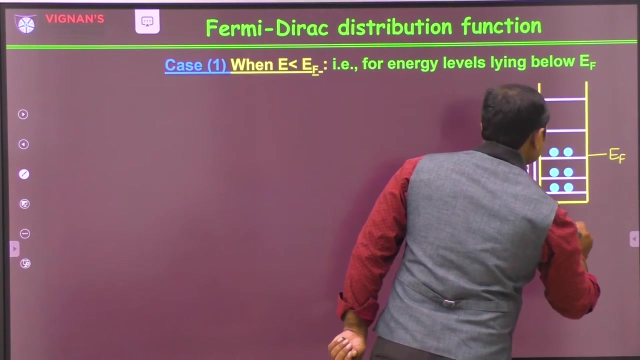 This is how the Fermi Dirac distribution function lies in, between 0 and 1.. Let us see some cases how the Fermi Dirac distribution function can give us information. Let us see a particular case, case number one, where the energy of the particle, the energy of the particle which we are finding, is less than EF. We know that this is the Fermi energy level. the highest field energy level at T is equal to 0. Kelvin is called Fermi energy level. 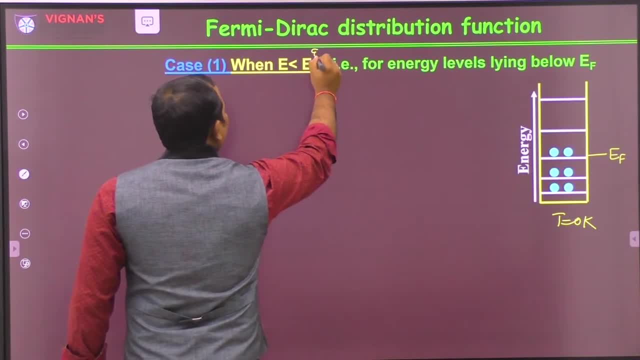 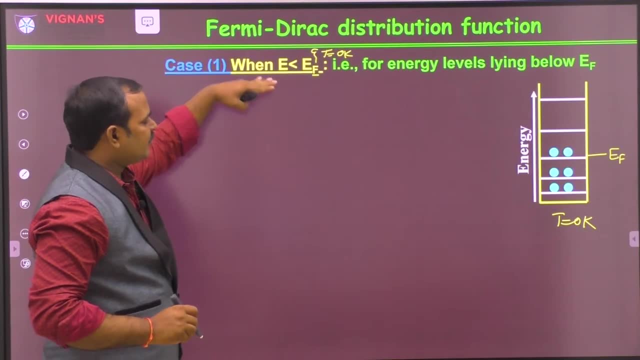 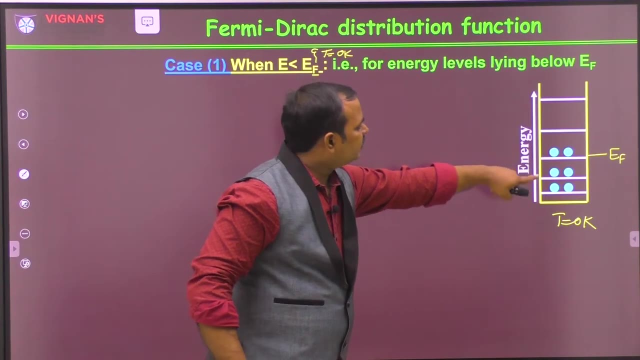 And also here the condition is: and at T is equal to 0 Kelvin. This is the case. that means below EF, below Fermi energy level, the probability of finding the particle. we are finding out Now that could be any energy level: 1,, 2,, 3, anything out of this: E1,, E2,, anything. 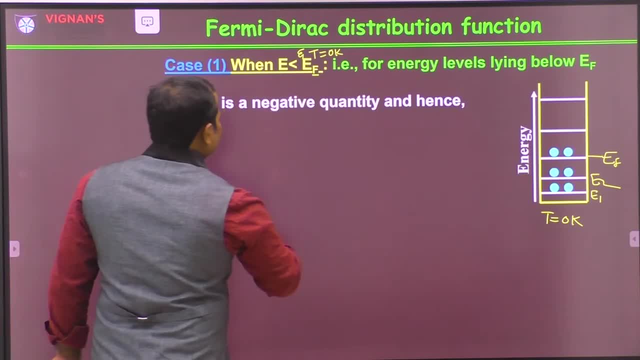 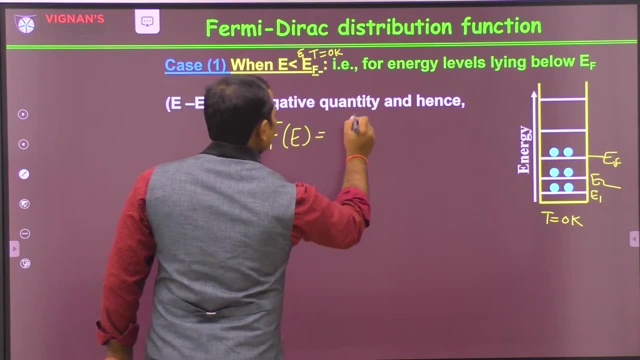 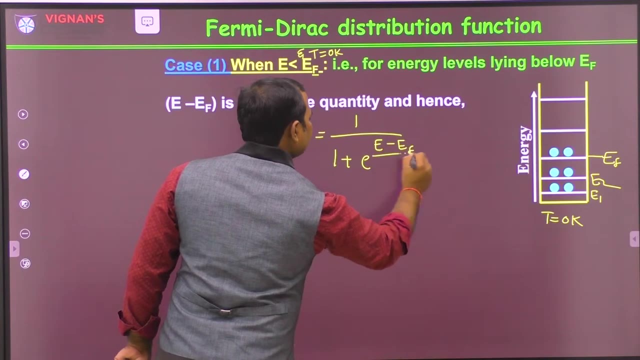 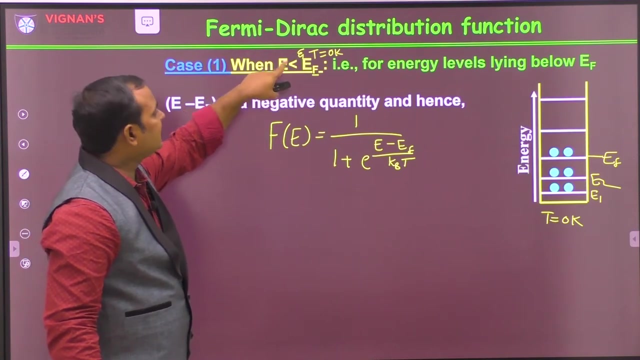 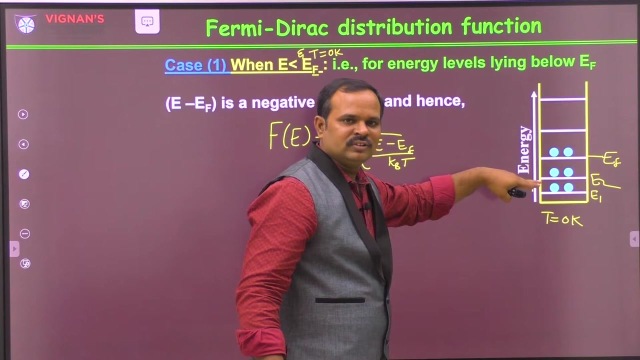 So here, if you see here the Fermi Dirac distribution, F of E is equal to 1 by 1 plus E power E minus EF by kB T. Now, when we consider the energy less than EF, that means somewhere some energy level. we are finding somewhere, either this or this which is below EF. what is the probability of finding the particle? 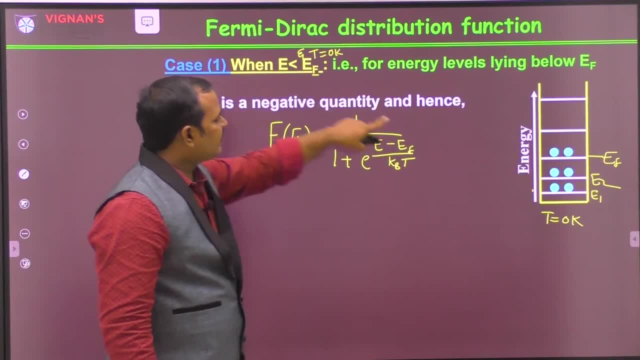 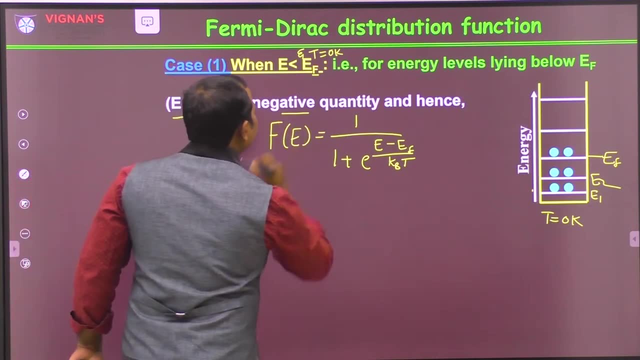 That is the meaning. Now, if EF is a higher, that means EF. the Fermi energy level is higher energy level. So E minus EF, that means E minus EF, would be a negative one. E minus EF would be a negative one. 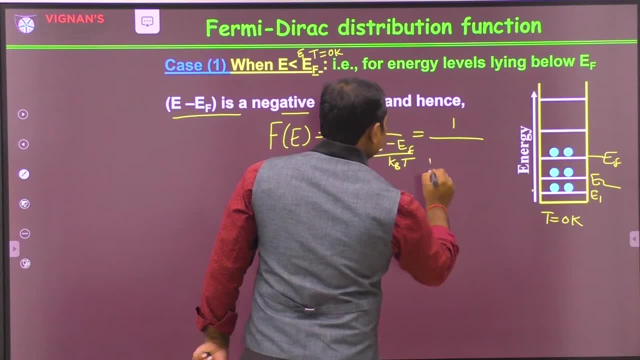 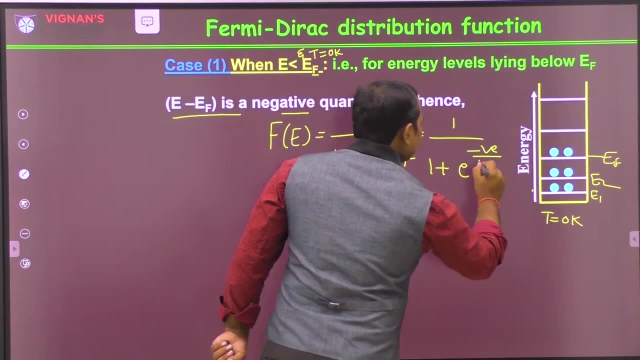 So we can write like this way here: 1 by 1 plus E power. This is a negative quantity. E minus EF will give a negative quantity by k into T is equal to 0, because we are considering a, T is equal to 0 Kelvin. 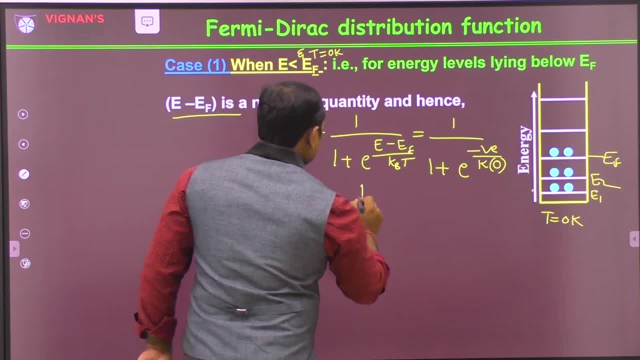 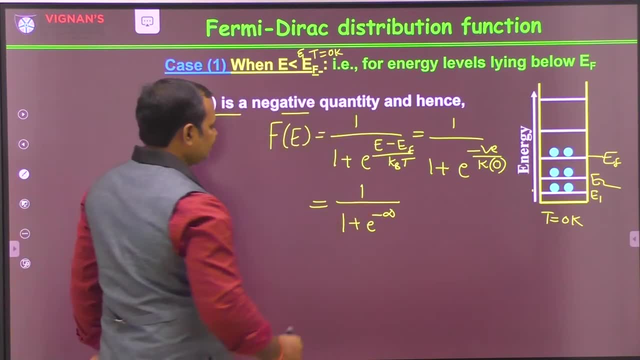 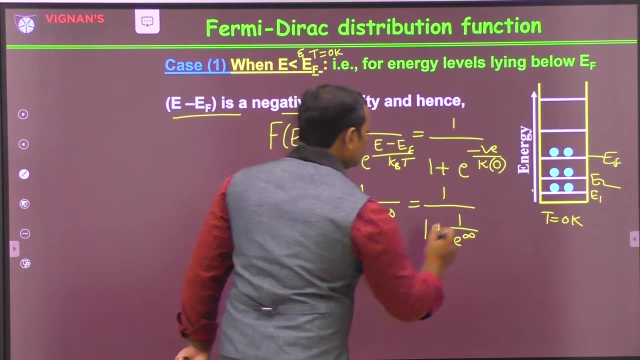 So what? we can write 1 by 1 plus E power minus infinity. So that means we can write 1 by 1 plus 1 by E power infinity, So which we can write 1 by 1 plus 1 by infinity. 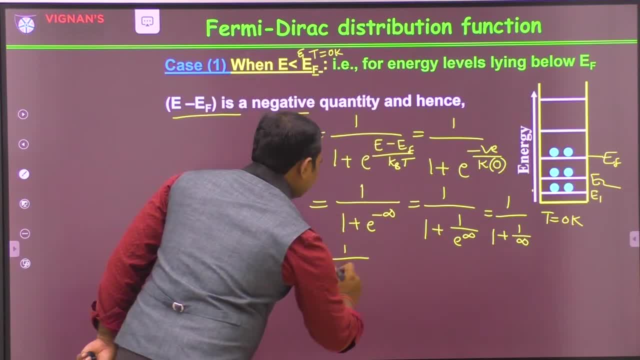 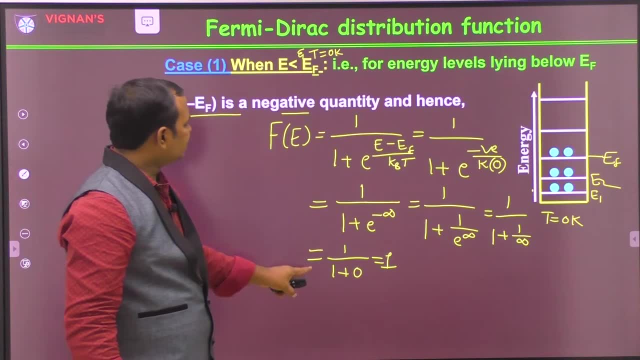 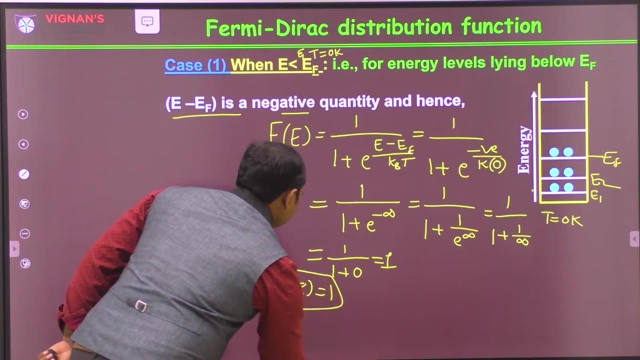 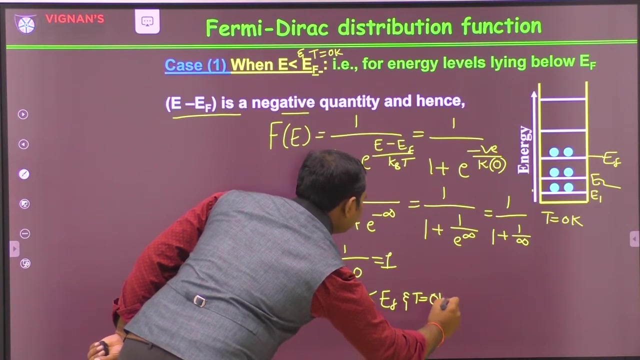 So 1 by 1 plus 1 by infinity is 0.. So 1 by 1 plus 1 by infinity is 0. Which is equal to 1.. The F of E is equal to 1.. So that means, if you see here F of E is equal to 1, when E less than EF at T is equal to 0 Kelvin. 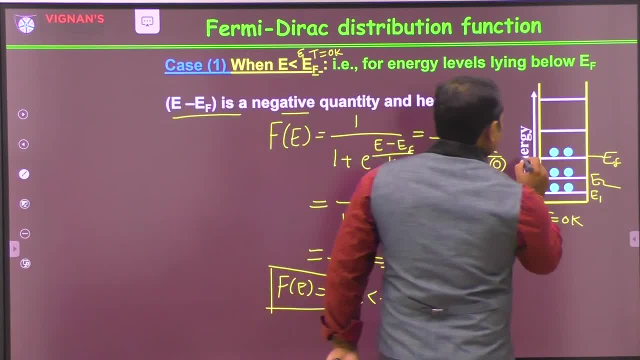 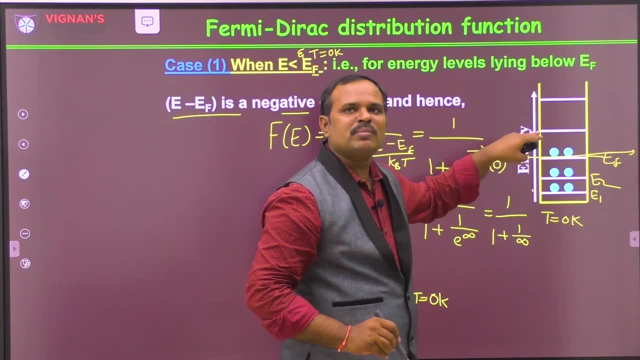 At T is equal to 0 Kelvin. That means this is the highest filled energy level, below which any energy level, if you find the probability of finding the particle, is always 1.. Because there is energy levels, there is electrons are already present. 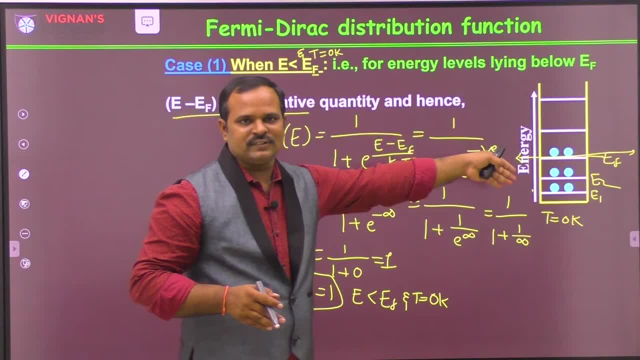 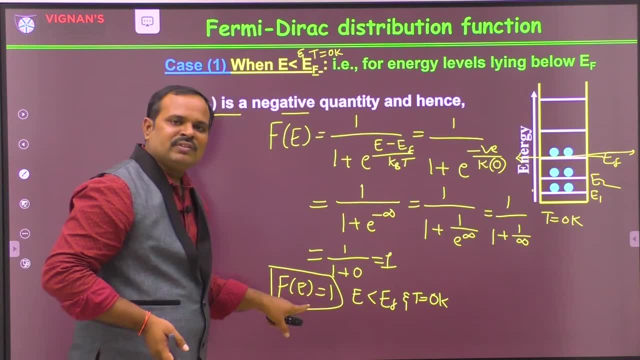 So if you use a distribution function on those energy levels, you always get 1, because there is already electrons are present in the particular energy level. That is the reason why you get F of E is equal to 1.. So now we can define Fermi energy level in this way. 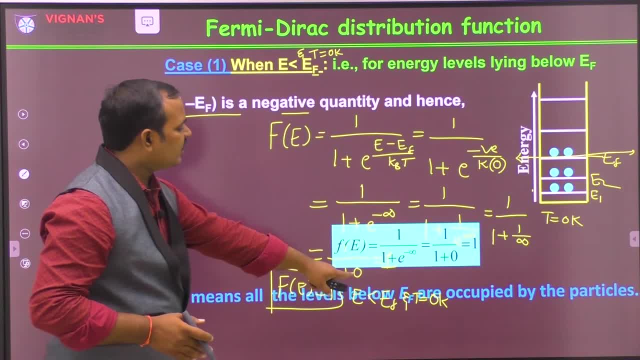 So that means all the particles below EF are occupied. All the energy levels are occupied by the particles. All the energy levels are occupied by the particles below EF. All the energy levels are occupied by the particles below EF. All the energy levels are occupied by the particles below EF. 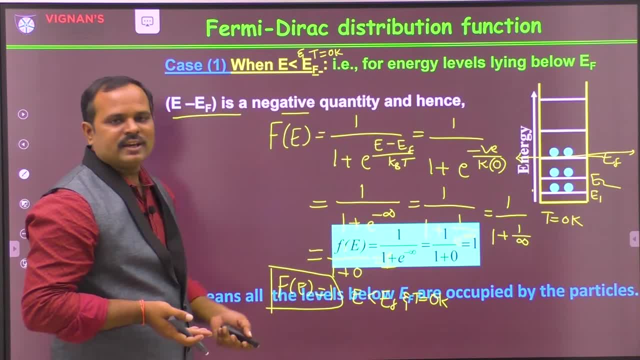 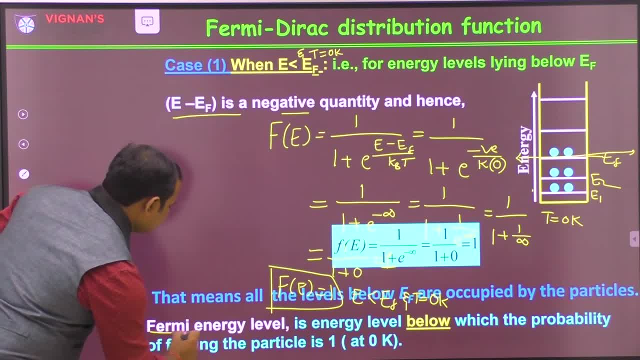 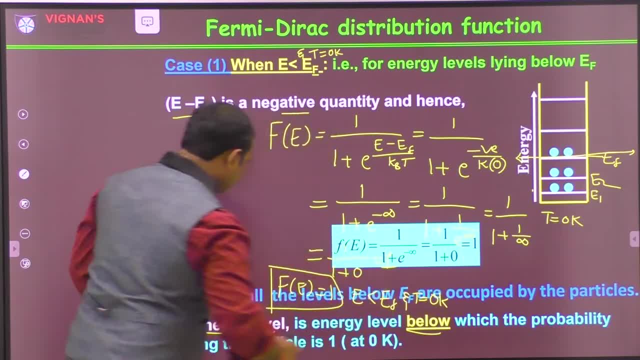 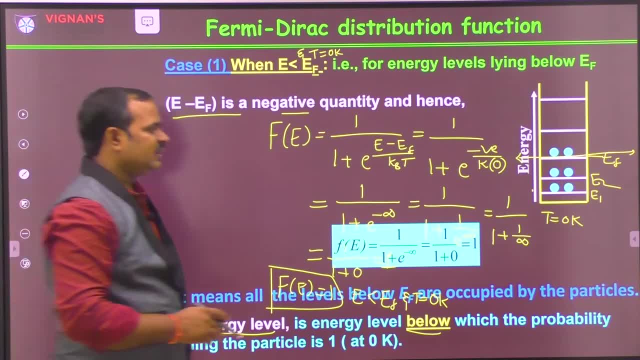 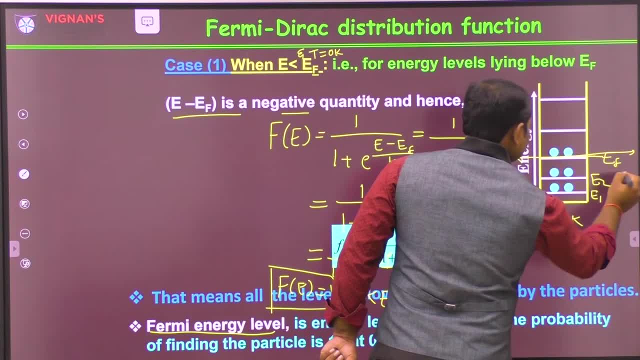 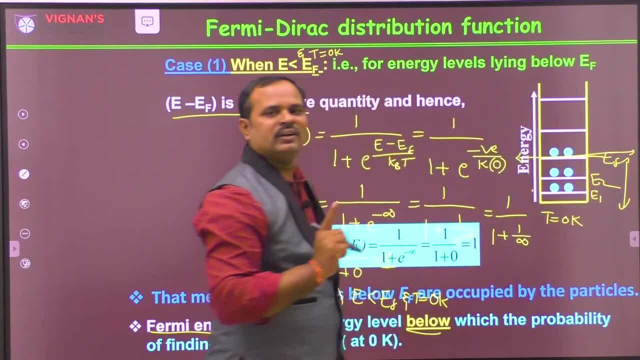 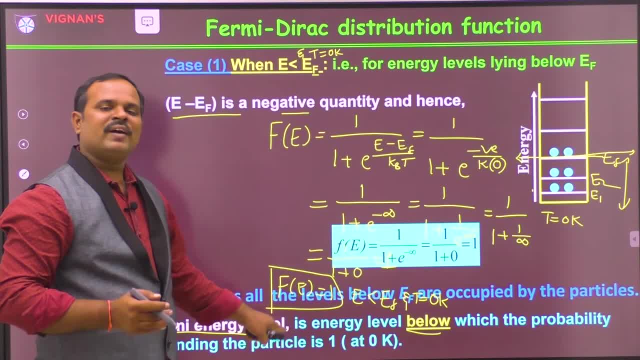 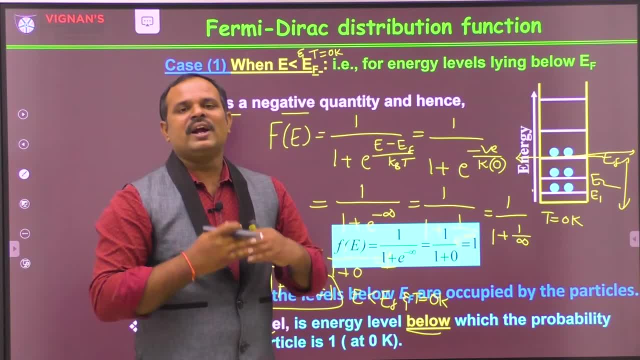 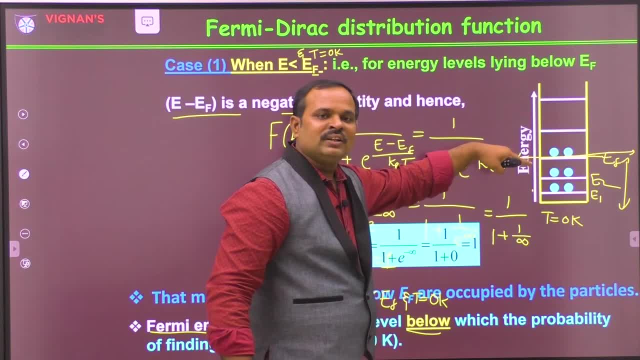 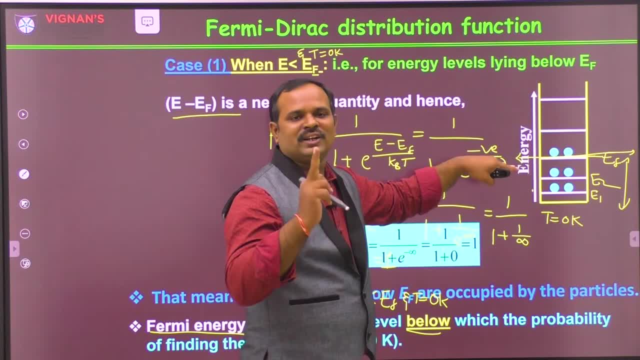 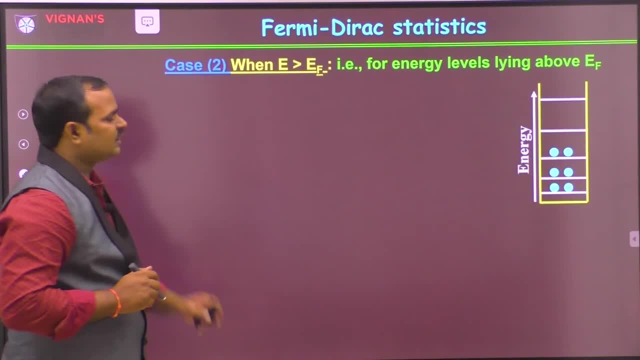 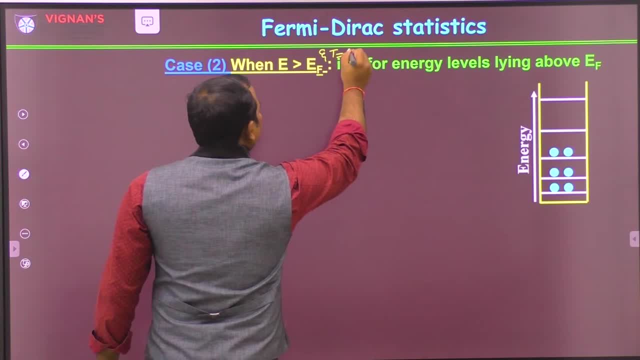 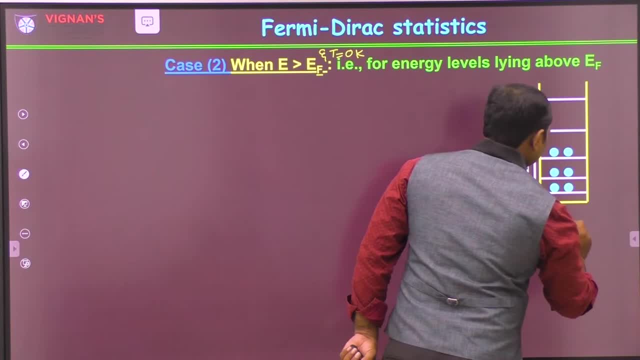 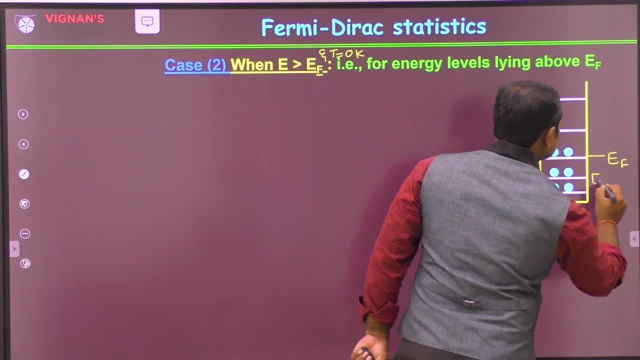 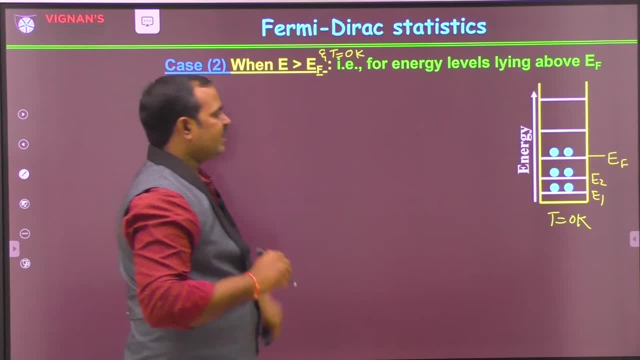 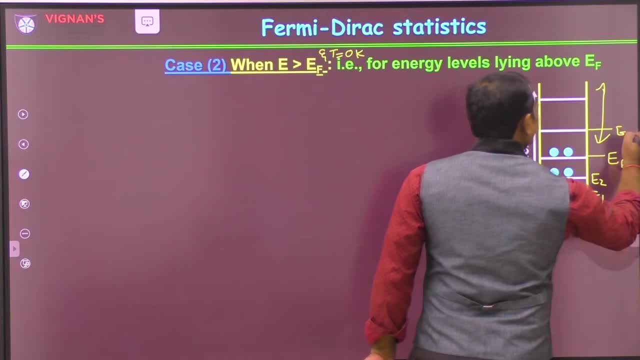 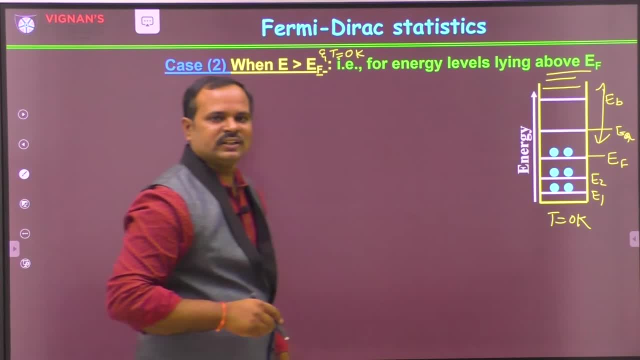 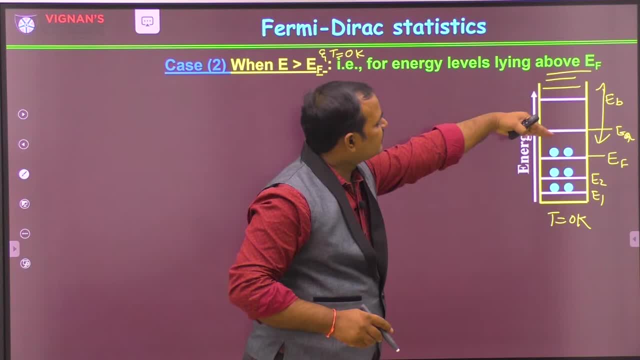 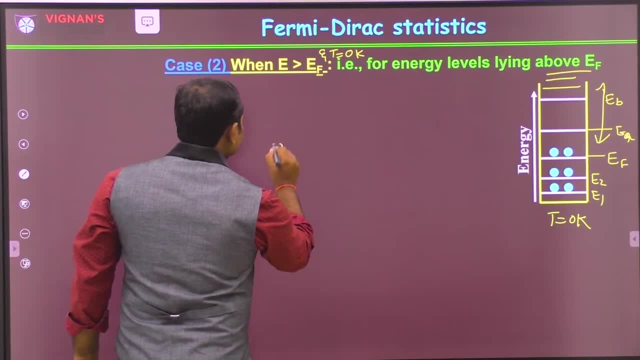 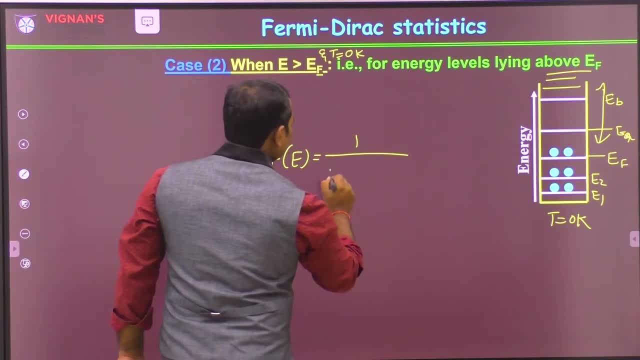 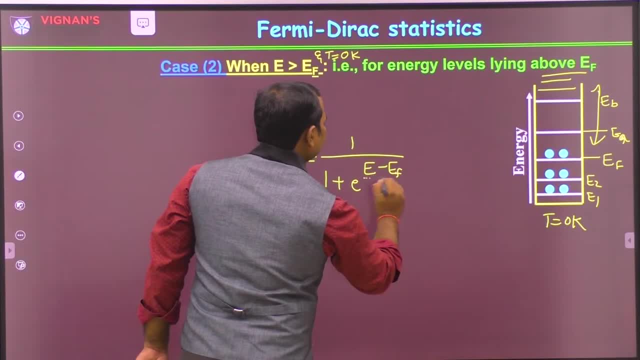 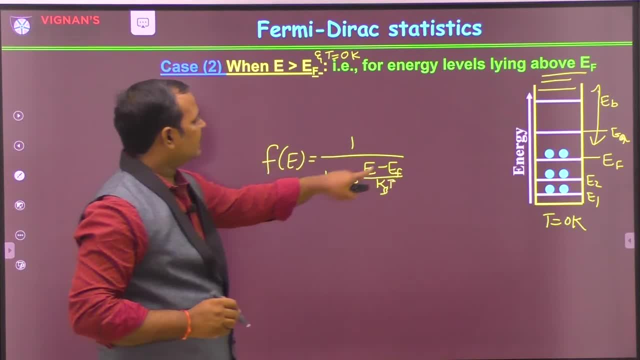 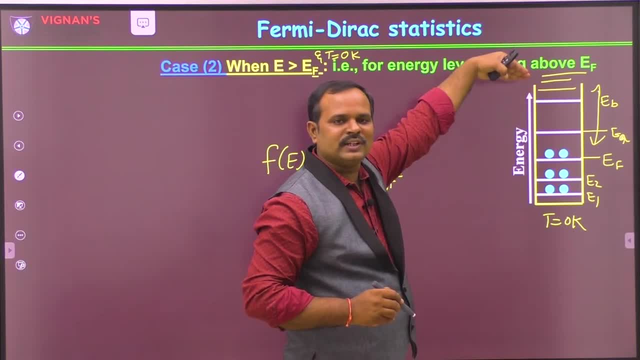 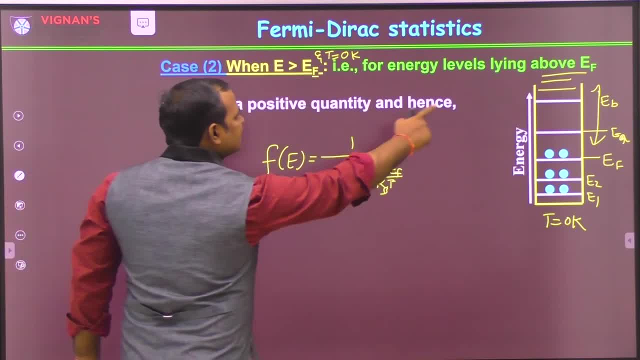 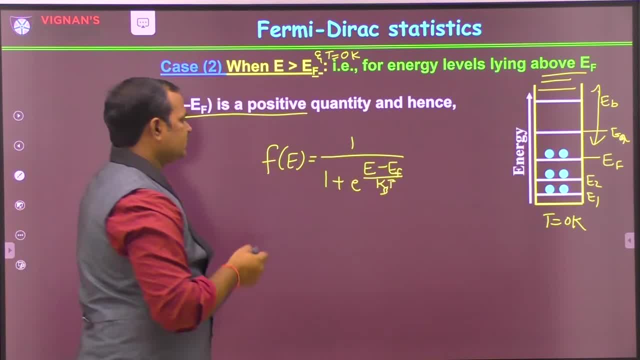 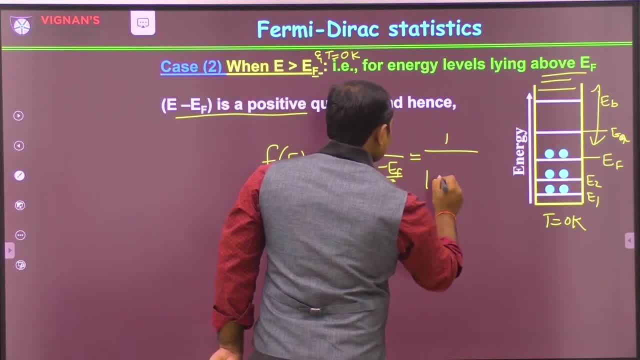 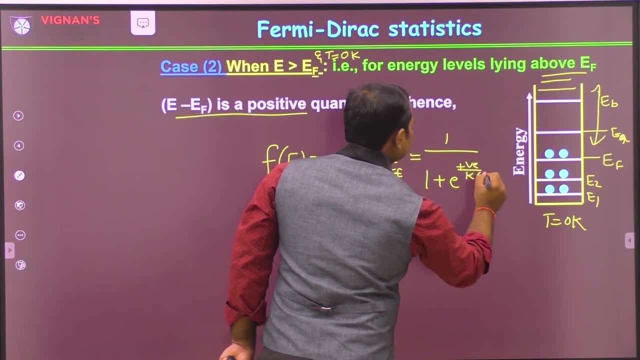 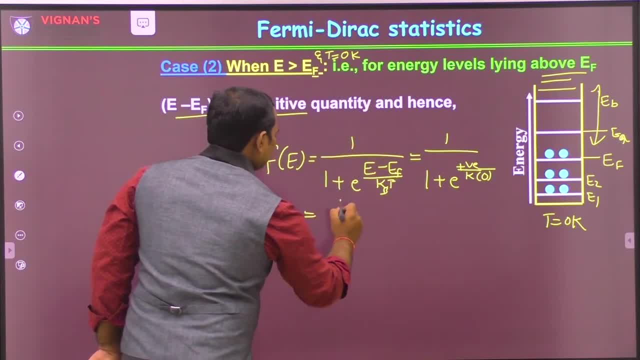 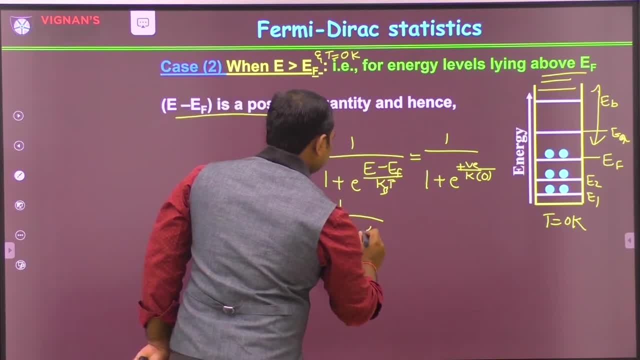 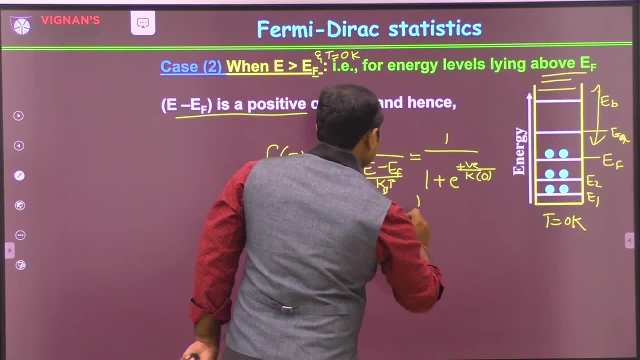 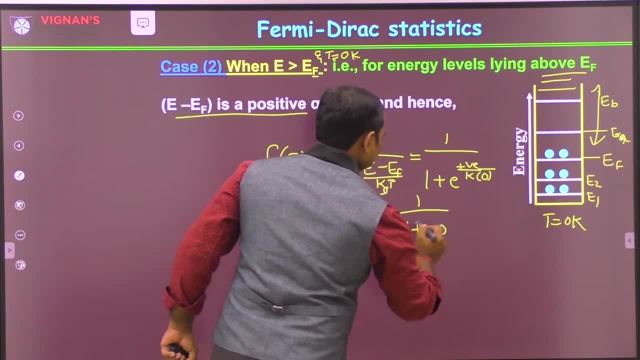 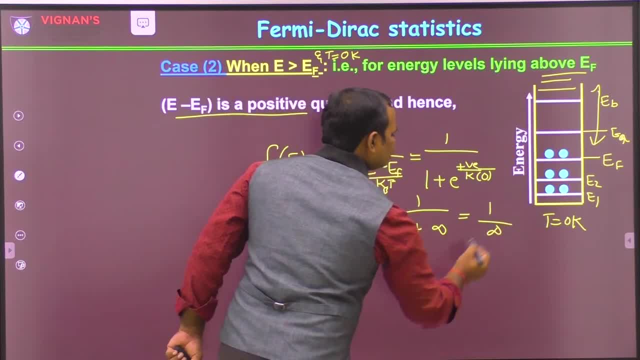 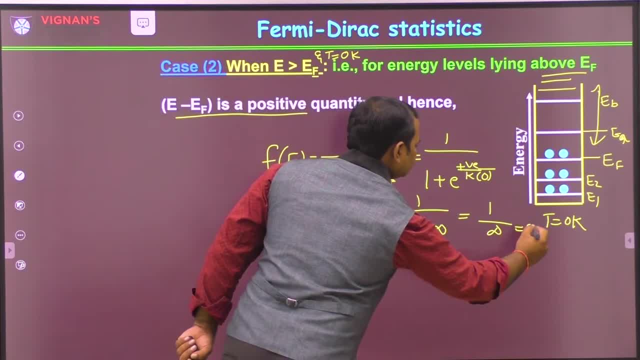 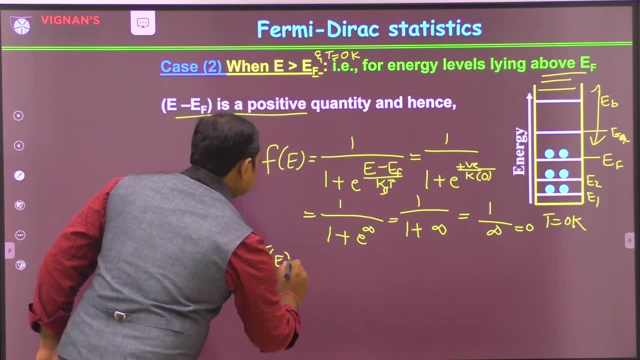 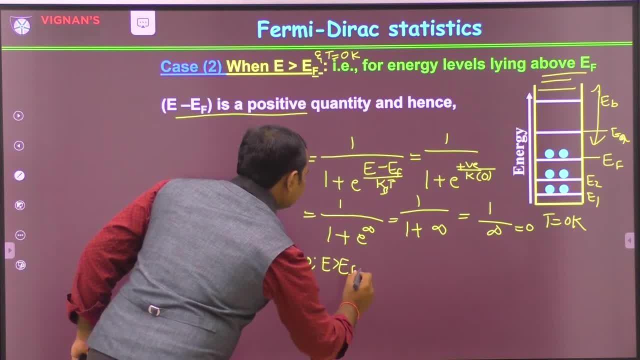 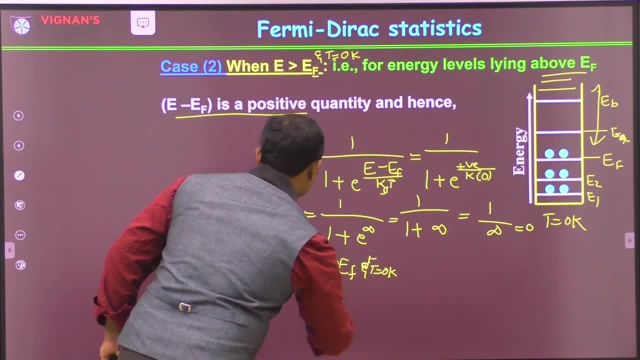 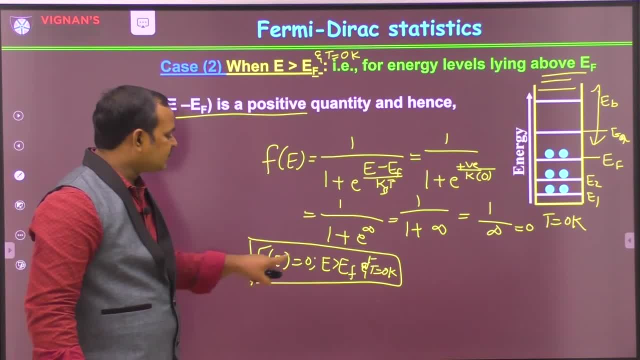 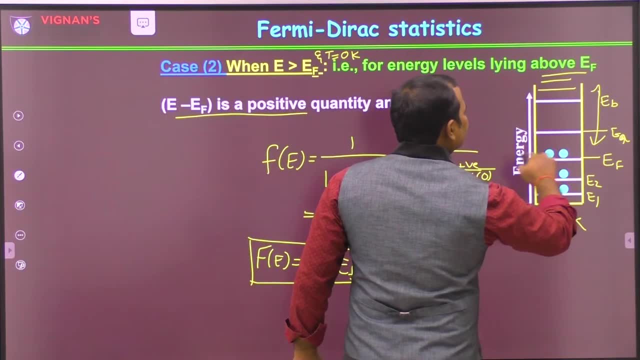 So the Fermi energy level is defined as at: t is equal to 0. So f of e is equal to 0. when e greater than f, That means the probability of finding the particle above Fermi level is always 0, because the Fermi level is the highest field. 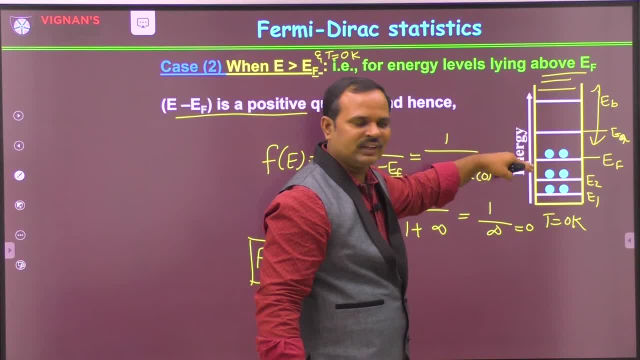 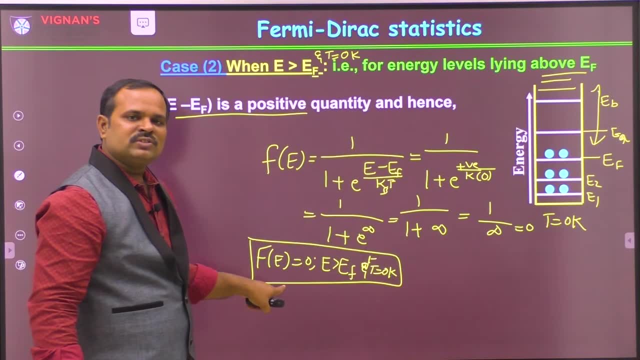 energy level below which all the electrons are filled. all the levels are filled. Above Fermi level, all the levels are empty. Obviously there is no electron. That is the reason why the Fermi-Dirac distribution function gives you a 0 value. So this is the second one. 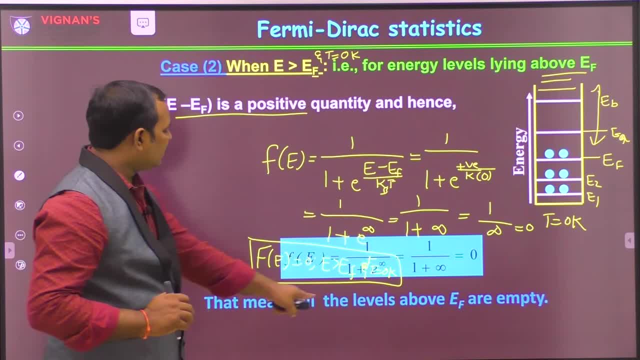 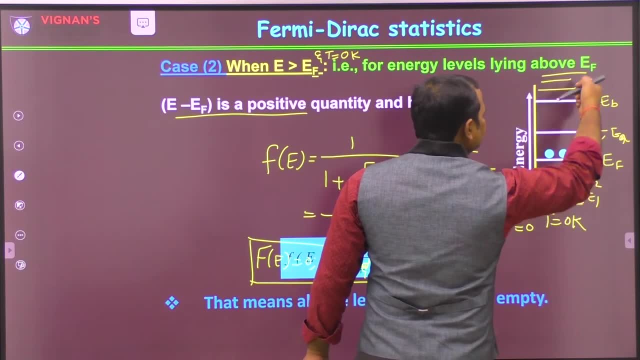 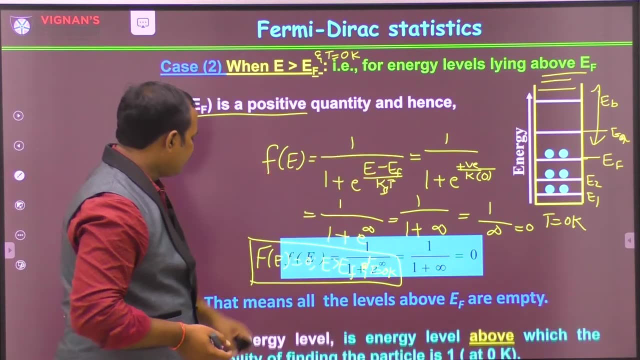 That means all like all the levels above e of r empty. That means this is the Fermi energy level, which all the energy levels are not occupied by the electrons. Now we can also define Fermi level with respect to this. Fermi level is energy level above which the 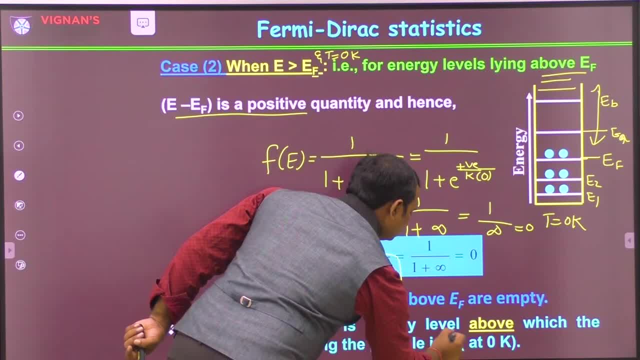 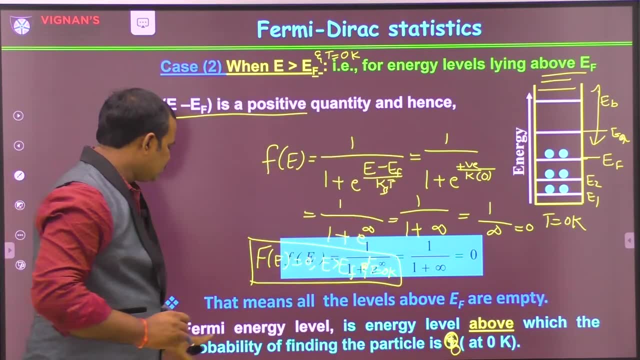 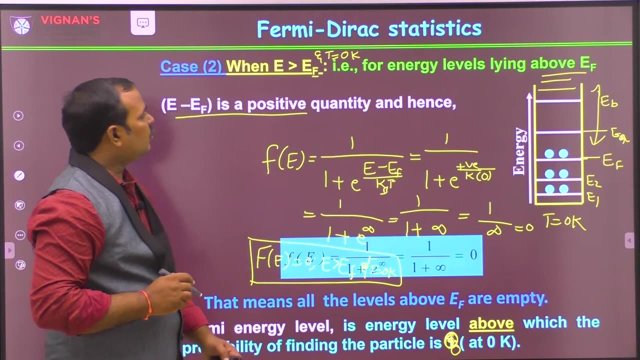 probability of finding the particle is zero. This is a zero Fermi level. is média result over given vielråd? OMG, energy level above which the probability of finding the particle is 0. That energy level is called Fermi energy level. Now, what happens at the Fermi level? Let us see that At the Fermi 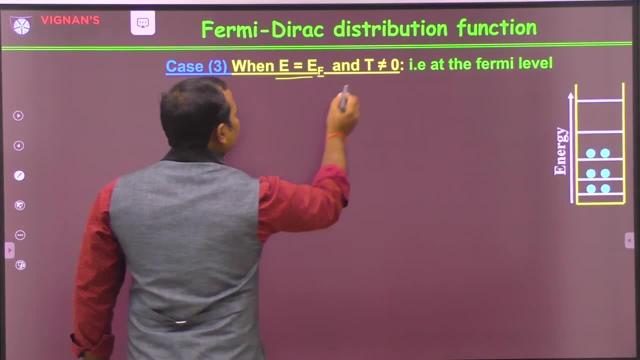 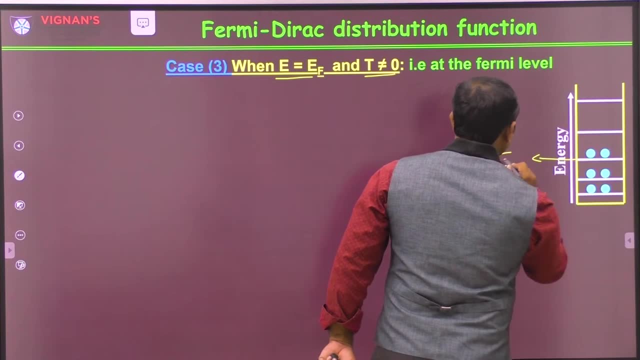 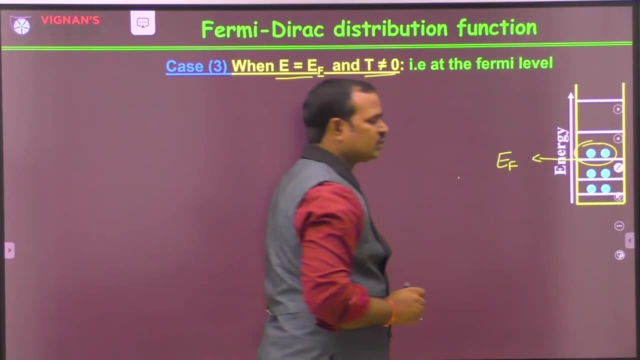 level that case 3,, E is equal to EF and T not equal to 0. This is not equal to 0 and this is the Fermi level EF. Now we are trying to find out. at this level, E is equal to EF, but here the 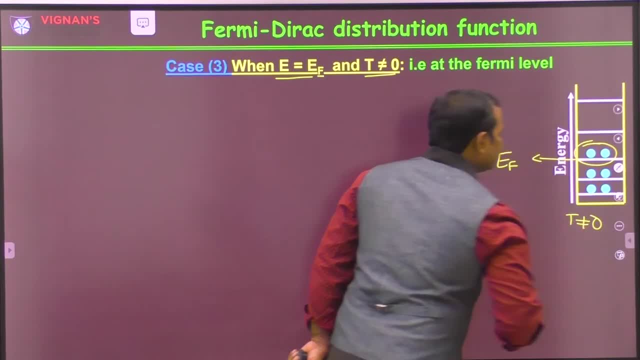 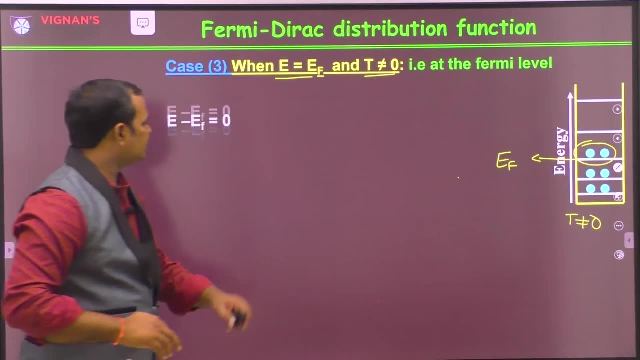 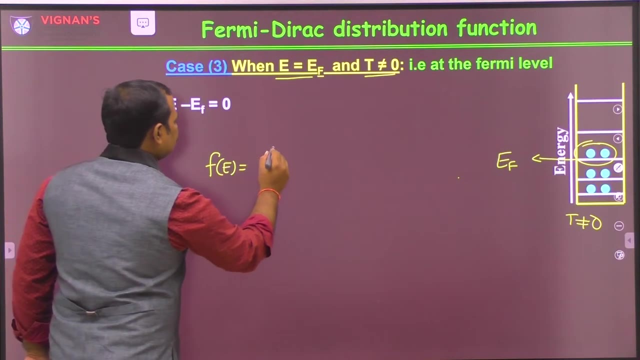 condition is T not equal to 0.. In the previous case we are considering, T is 0, that means temperature is 0. What happens, Let us see. So Fermi drag distribution function E minus F is equal to 0.. The Fermi drag distribution function F of E is equal to 1 by 1.. 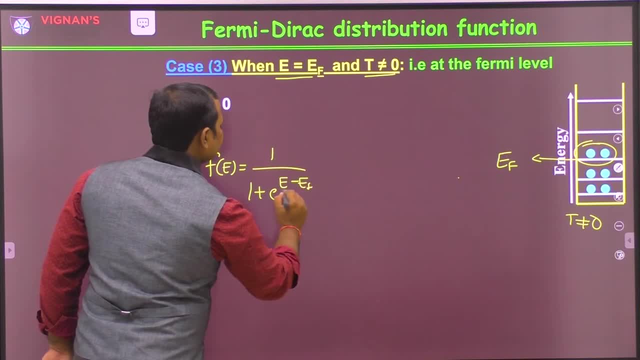 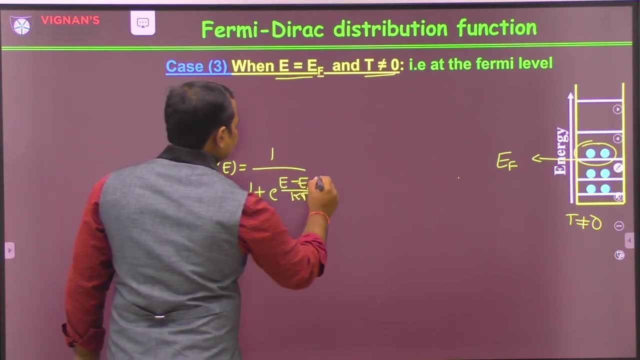 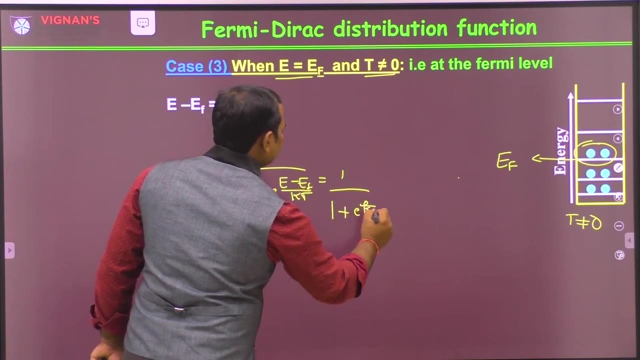 E power: E minus EF by KT, T is not equal to 0. now E minus EF is equal to 0. So what we can do here, We can do 1 by 1 plus E minus EF is 0.. So E power 0 by KT, which we can write 1 by 1 plus. 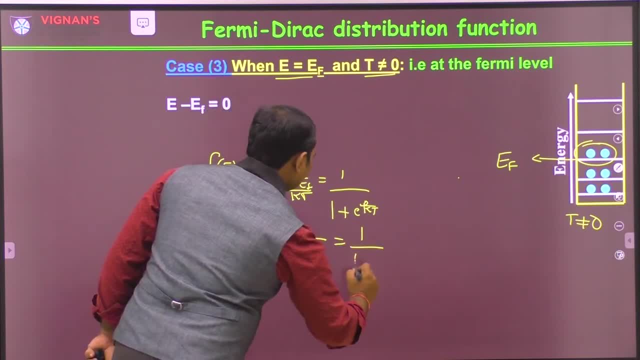 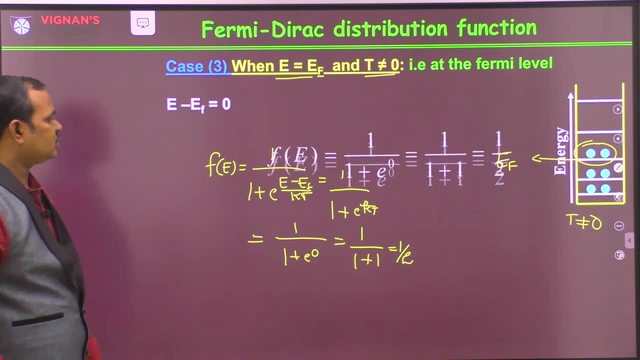 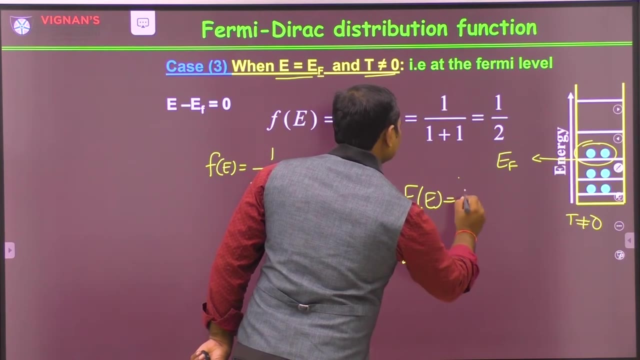 E power 0,, which we can write 1 by 1 plus E power 0, is equal to 1, which is equal to 1 by 2, like this way 1 by 2.. So that means F of E is equal to 1 by 2, where E is equal to EF. 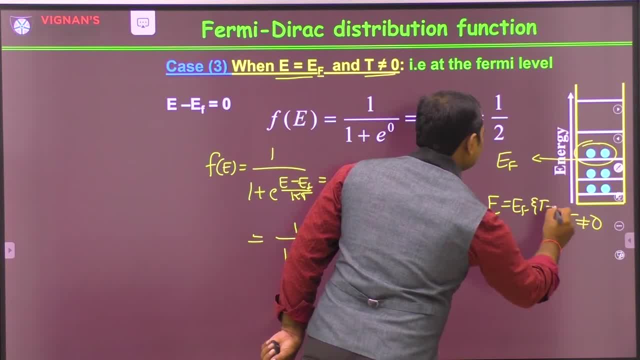 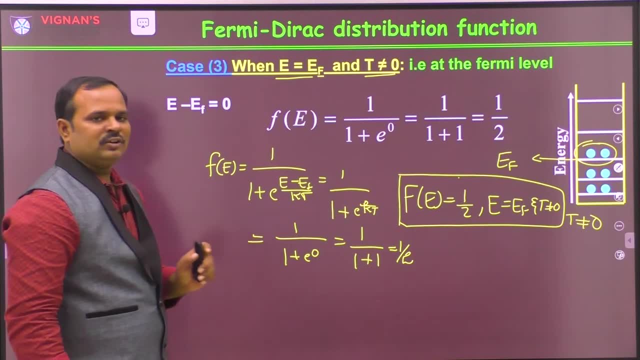 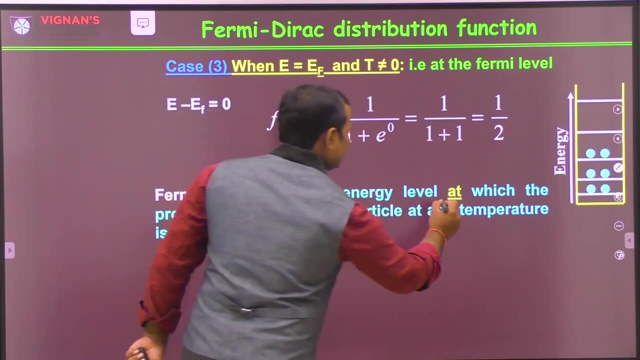 and T not equal to 0.. This is the third condition. So now from this one we can also define Fermi level. So Fermi level is the energy level At which at Fermi level at which the probability of finding the particle at any temperature is. 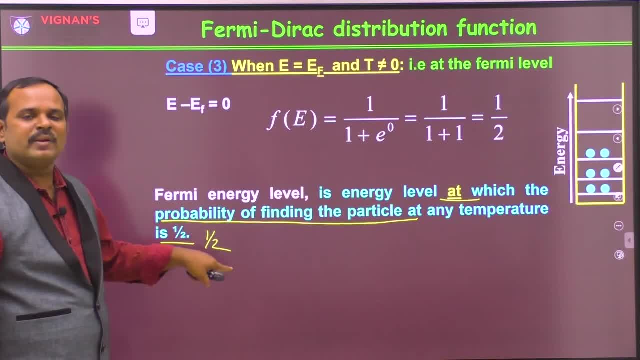 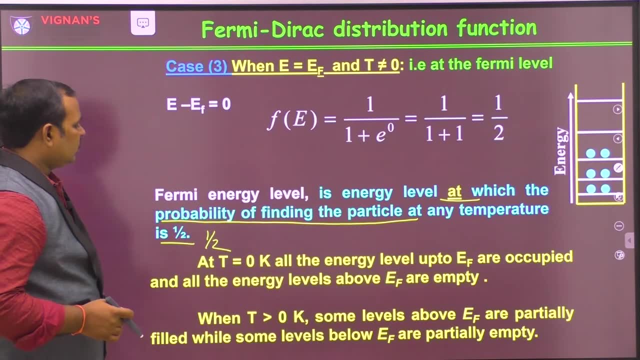 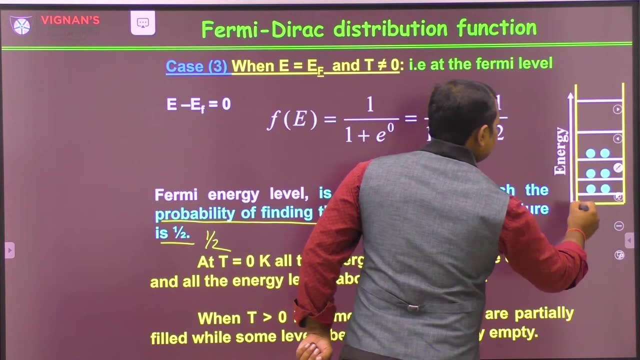 half. That level is called Fermi energy level. Fermi energy level has a lot of different definitions. Every definition is correct. So at T is equal to 0 Kelvin, all the levels up to EF are occupied. That means until the Fermi energy level, all the energy levels are occupied. 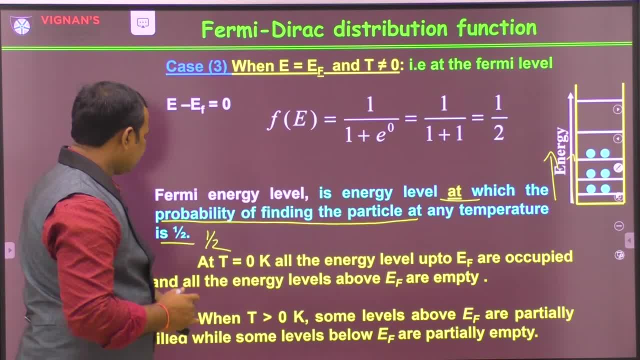 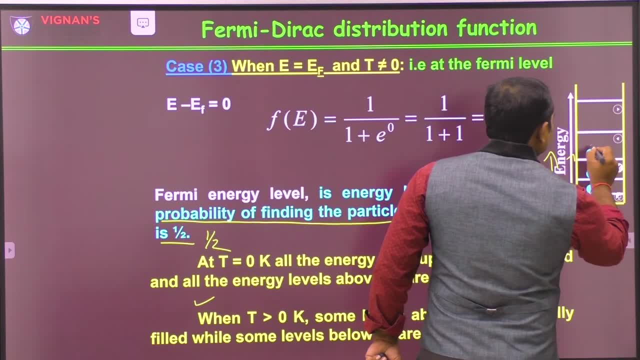 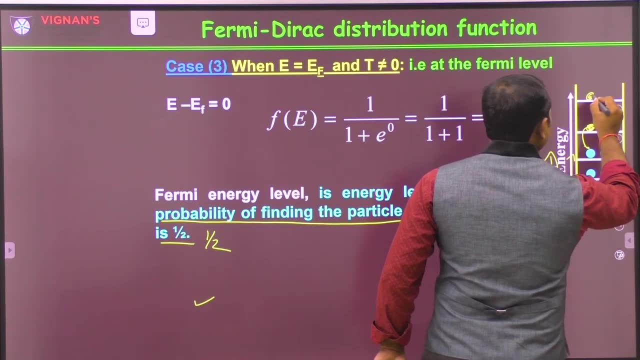 and all the energy levels which are above EF are empty And at T greater than 0 Kelvin, some of the energy levels above. now you are applying temperature. So what happens? Because of the temperature, the electrons will take energy and goes to higher energy state. So 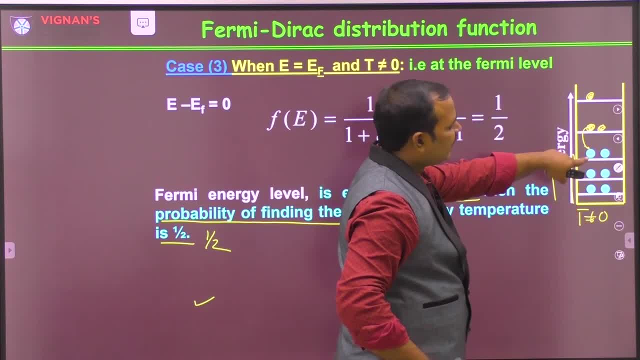 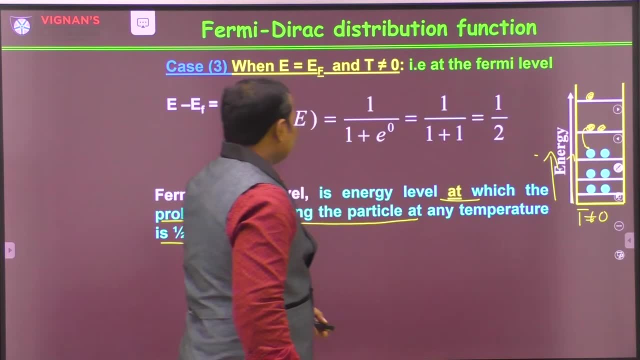 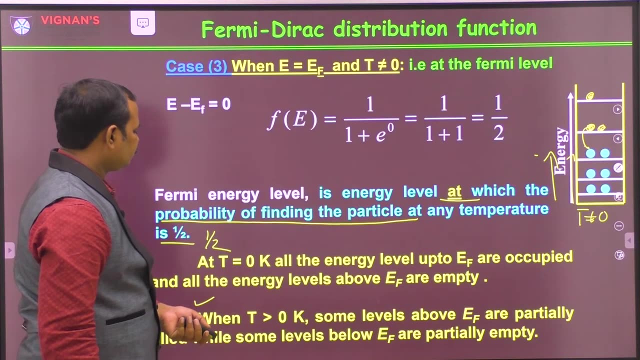 and T is not equal to 0,. what happens? Some of the electrons will get energy from the top energy levels. that means closer to EF and then goes to higher energy levels. So you have a change in. you have a change in Fermi energy. Now let us draw the graph. 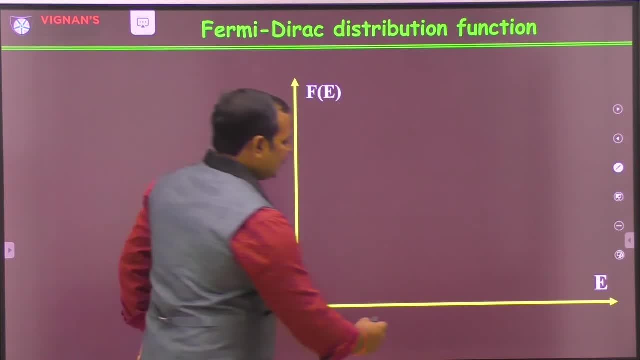 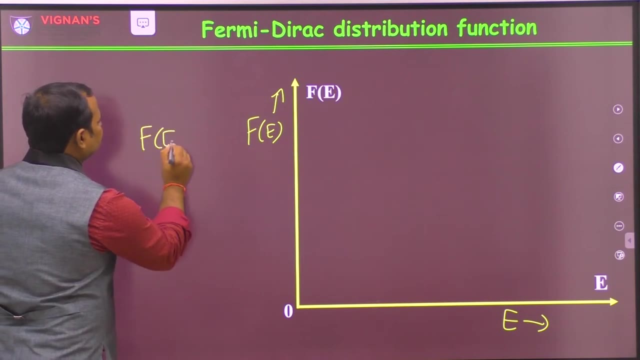 between Fermi energy versus energy. This is the energy of the system and this is the Fermi Dirac distribution function. how it is varying, We know. we know there are. the conditions are: F of E is equal to 1.. 1. 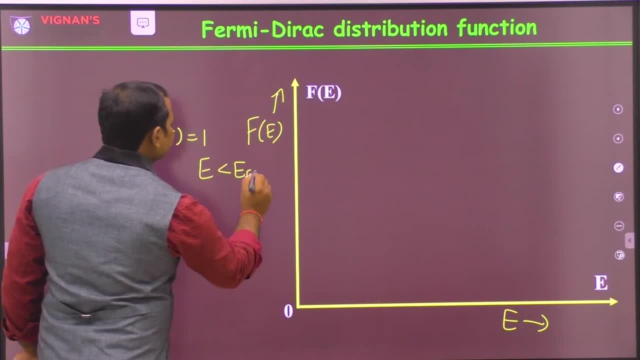 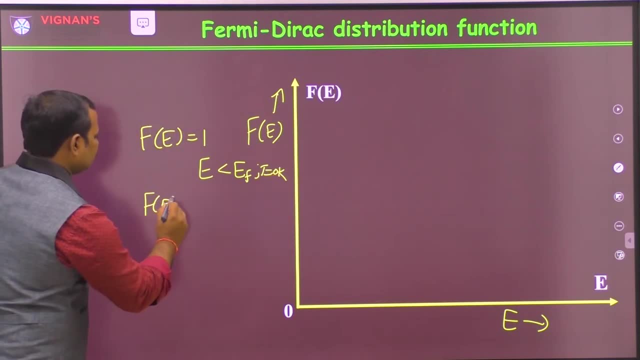 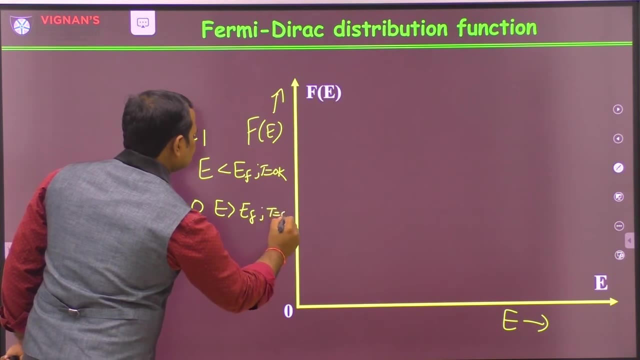 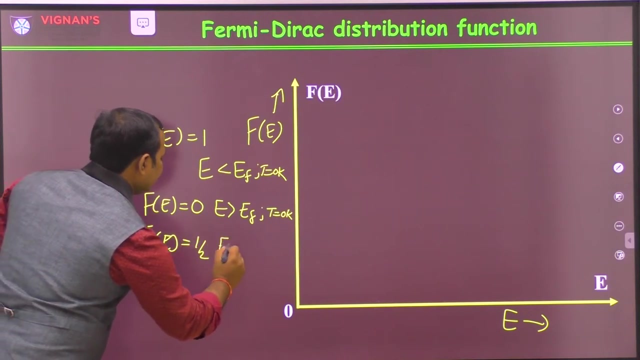 Then E less than EF and also T is equal to 0 Kelvin. The second condition is: F of E is equal to 0, E greater than EF. This is also at a. T is equal to 0 Kelvin and F of E is equal to 1 by 2, where E is equal to EF, but here T not equal to 0. 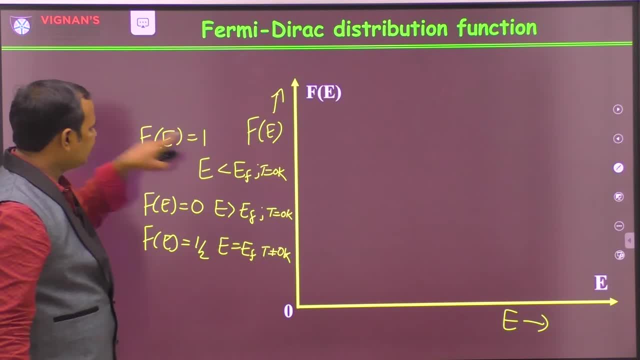 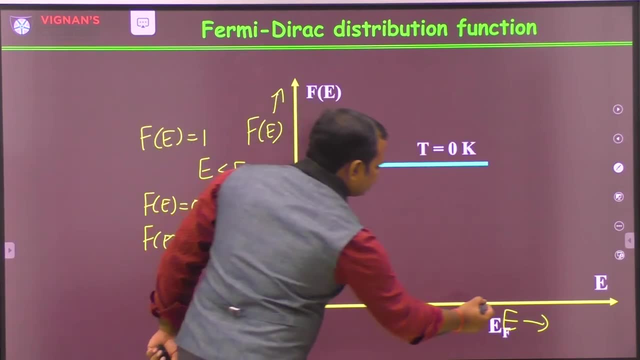 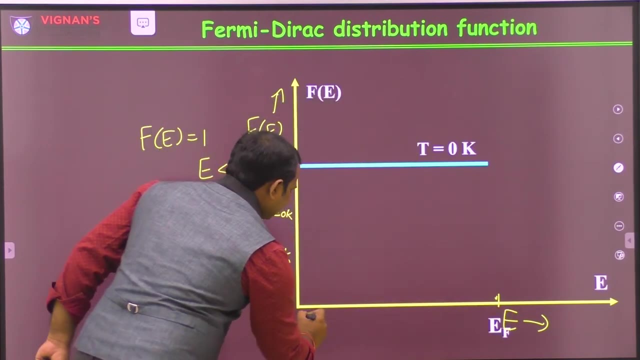 That means there is some temperature we apply. Let us fill this in the graph Now. if you see here E less than EF. there may be somewhere we are considering this is the Fermi energy level, somewhere, So below EF. that means this is the smaller energy compared to EF. 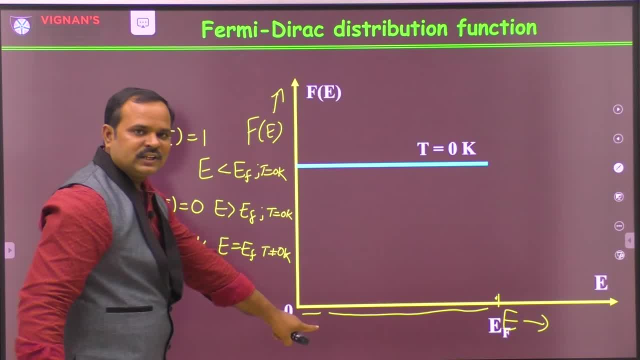 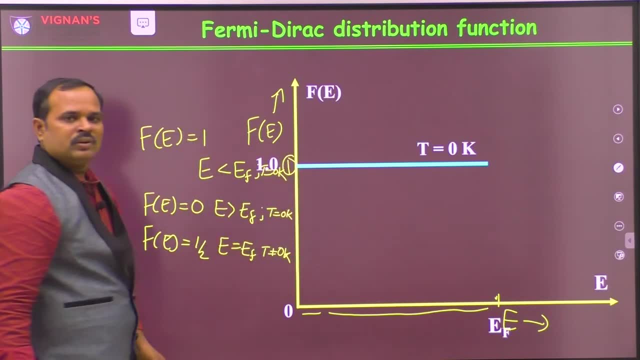 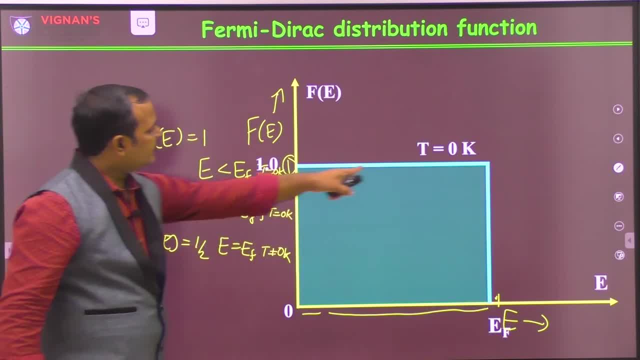 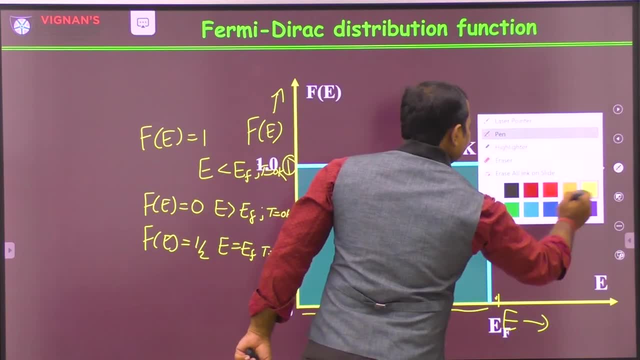 1.. That is the reason why you have line here and at E is Now, until this point, this reason- the probability of finding the particle is 1, and after that the probability of finding the particle is 0. So you have 0. whether you write it or not, this is 0. So no need. 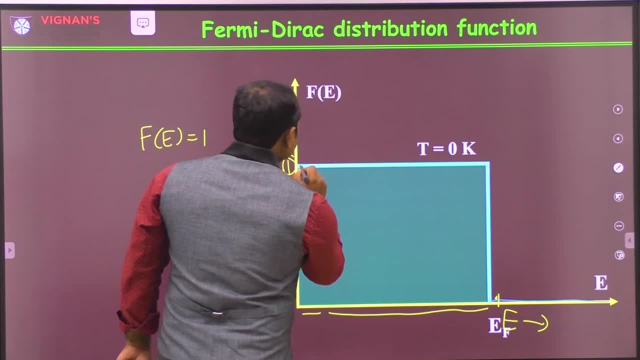 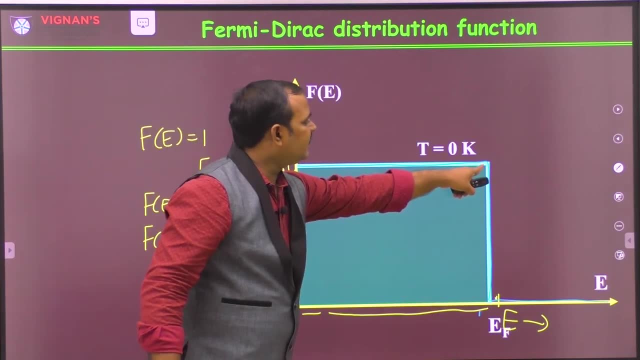 to write. That is the reason why you can see this is a step function. This is a step function 1. 1. 1. EF. suddenly, until E is equal to EF, you have a probability of finding the particle is 1.. 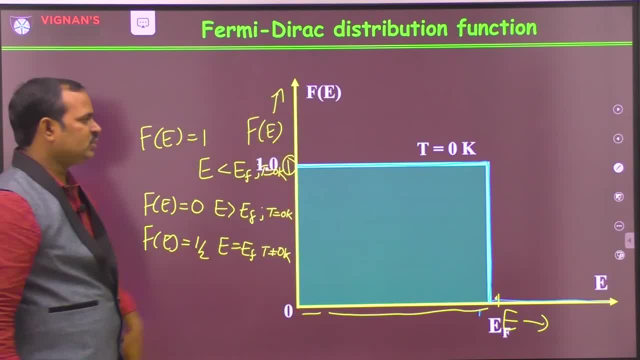 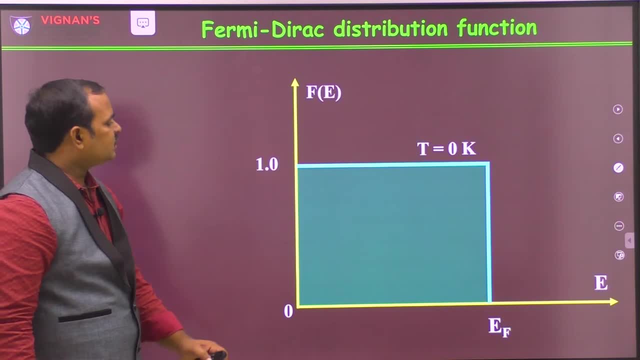 Now at T is equal to EF- what is the thing? But it is not. T is equal to 0.. All these graph is for: T is equal to 0 Kelvin, But T is equal to not 0 Kelvin. this is how it look like. 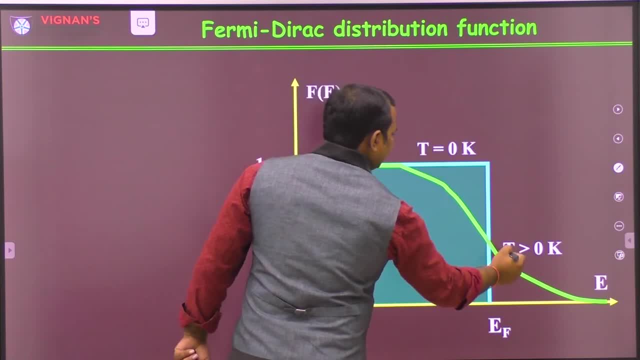 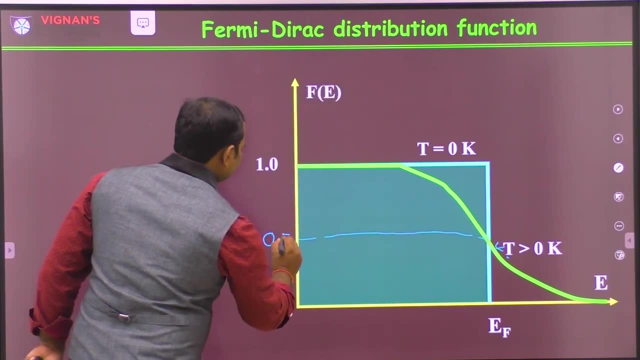 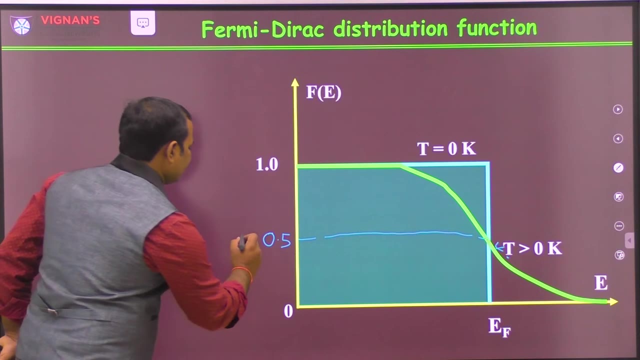 You can see here, at T is equal to this. is the T not equal to 0 Kelvin? At E is equal to EF. you have at Fermi level. you only have half of the probability, that is 0.5, but we 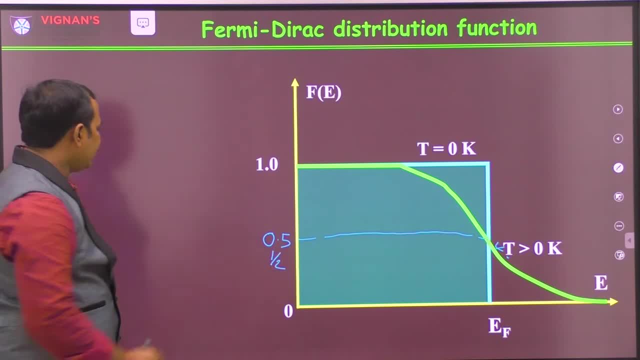 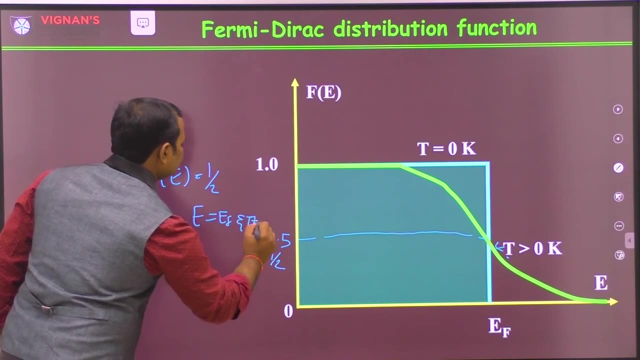 can also write: this is 1 by 2.. This is the condition here. F of E is equal to E. F of E is equal to 1 by 2, where E is equal to EF at T not equal to 0 Kelvin. 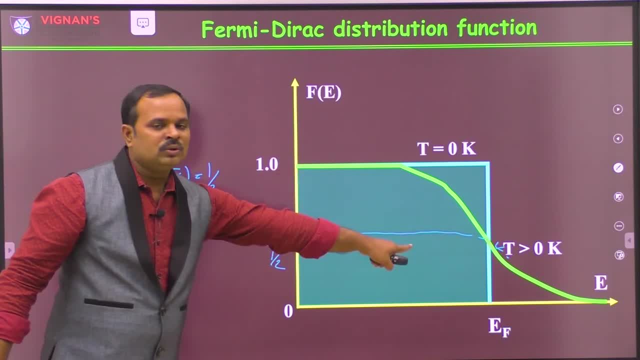 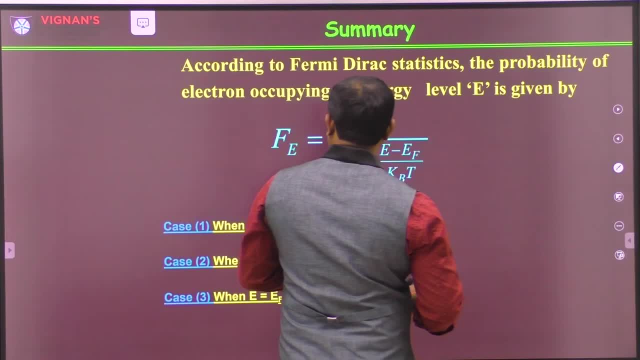 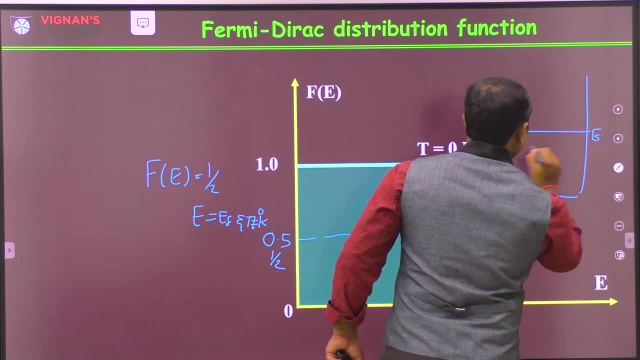 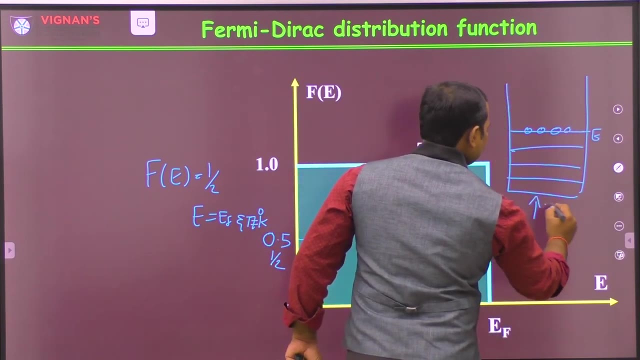 function is changing. This is because, if you see here, this is the Fermi energy level, EF. until these energy levels, all of them, are filled. Now, this is the Fermi energy level. Now, when you increase the temperature, what happens? These are the empty energy levels. 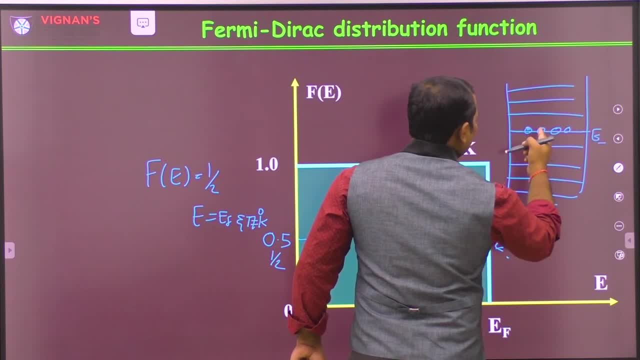 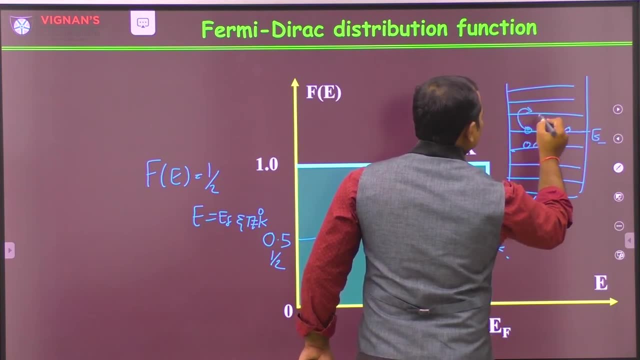 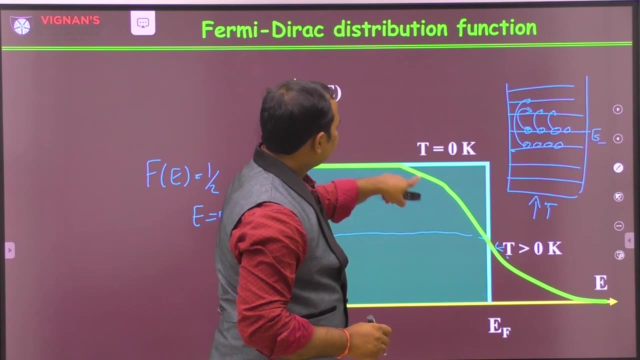 So when you increase the temperature, the electrons which are actually above, closer to the Fermi level- either this level or this level electrons- will gain energy and goes to next energy levels. So that is the reason why you can see there is a decrement here. 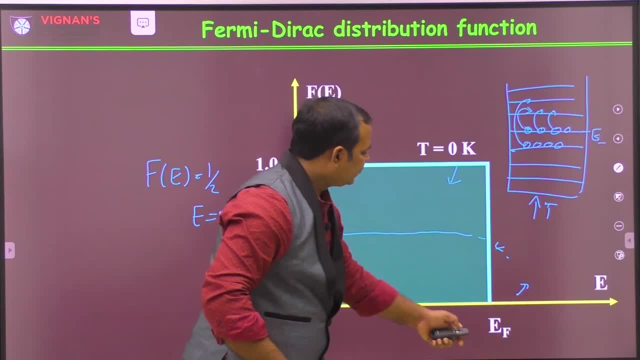 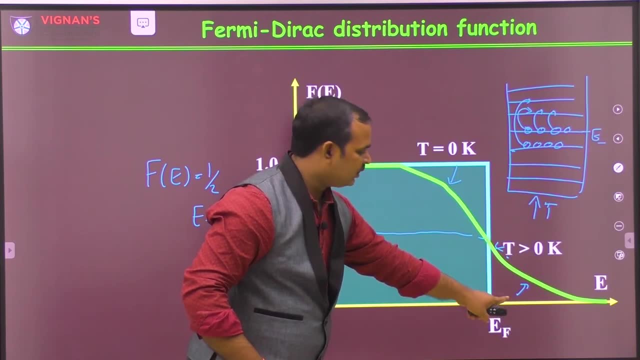 and there is an increment here Above EF. previously there is no occupation of energy. The probability distribution function is 0. But at T greater than 0 Kelvin there is a some probability of finding the particles. That is because at T greater than 0 Kelvin. 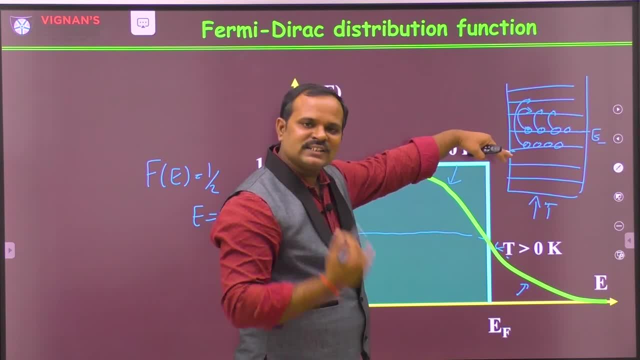 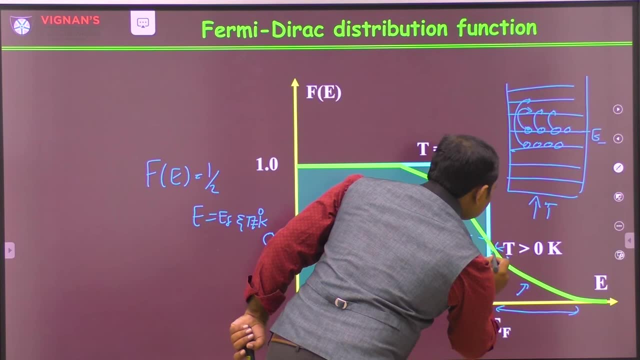 then some of the electrons closer to Fermi level takes energy from the heat energy and exalt to higher energy level. That is the reason why, above EF, you have some probability of finding the particles At the same time here, the probability of finding the particle. 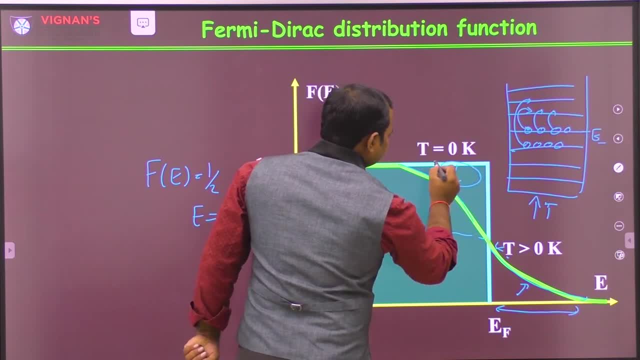 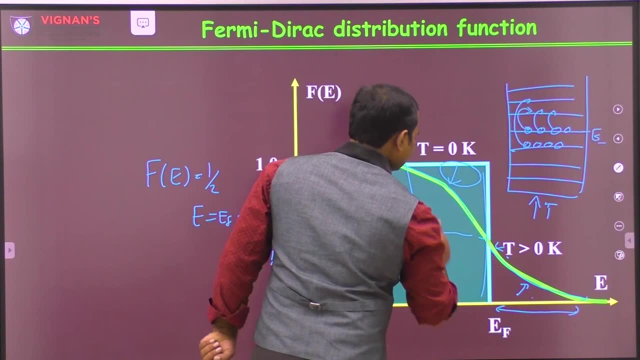 is decreasing. That is because these energy levels from here to here, these energy levels are moving to here, From here to here. That is the reason why you have a decrease in the Fermi Dirac distribution function and here you have an increase in the Fermi Dirac. 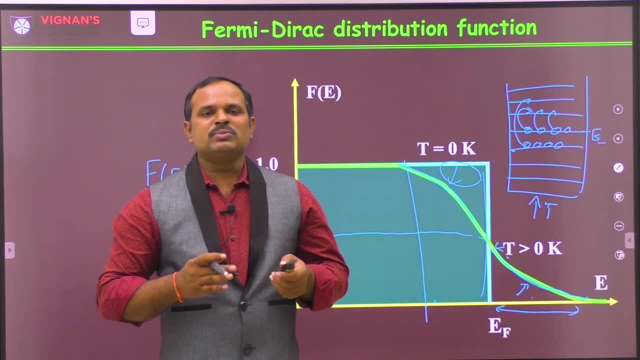 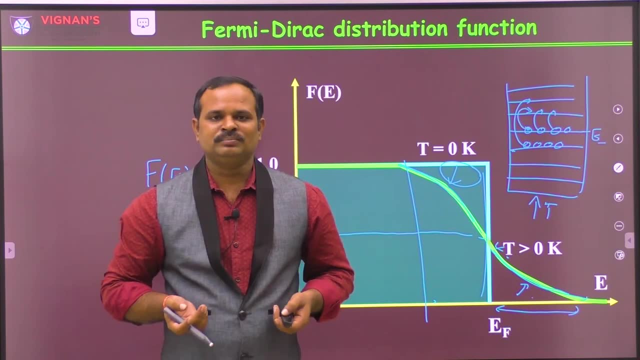 distribution function. This is how the Fermi Dirac distribution function can give us information about how the particles are being occupied in a particular energy level. The cases are: T is equal to 0 Kelvin. it can give you T greater than 0 Kelvin also. it can give you: